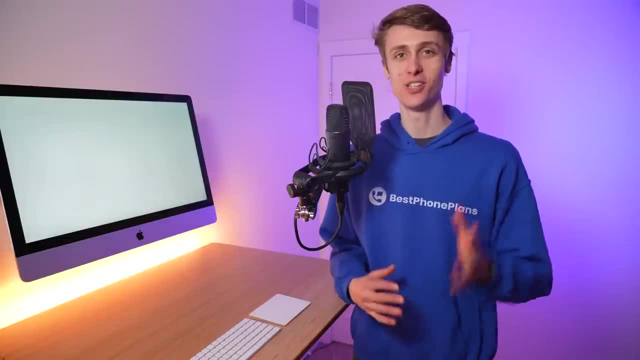 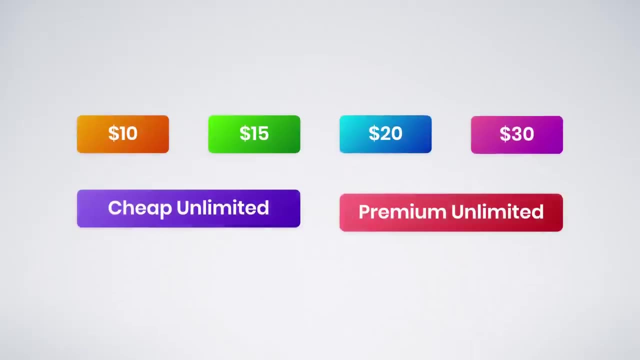 In this video, I'm covering the best cell phone plans for 2021.. I'll be covering the best plans on Verizon, AT&T and T-Mobile, and I'll be covering plans ranging from $10 to $15 to $20 to $30, and even the best cheap and premium unlimited data plans. These plans will deliver. 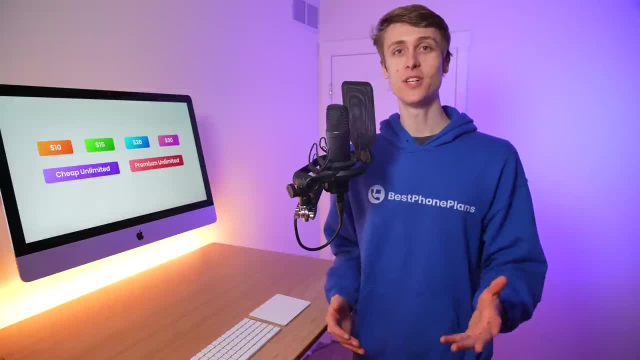 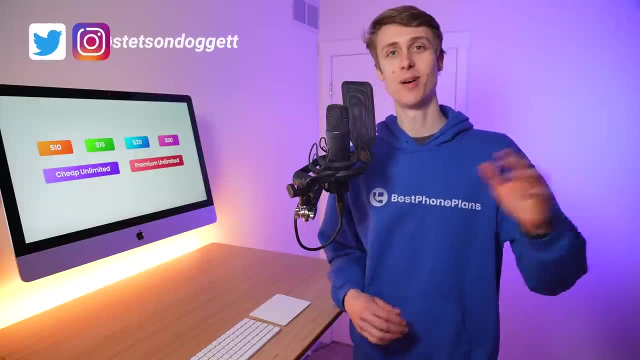 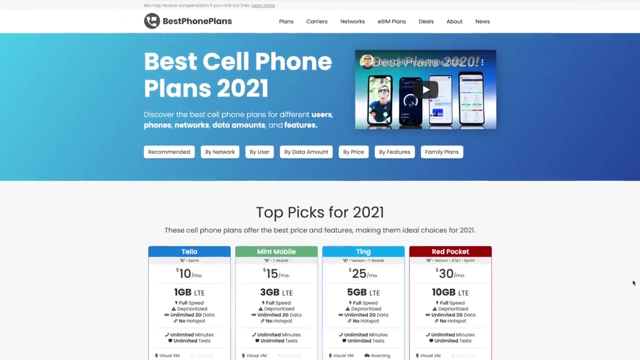 the best value for your dollar and include many of the features you love, like voice over, LTE, Wi-Fi calling, mobile hotspot and more. Hi, I'm Stetson and I've been reviewing cell phone plans since 2015.. I even designed and built bestphoneplansnet to help make it. 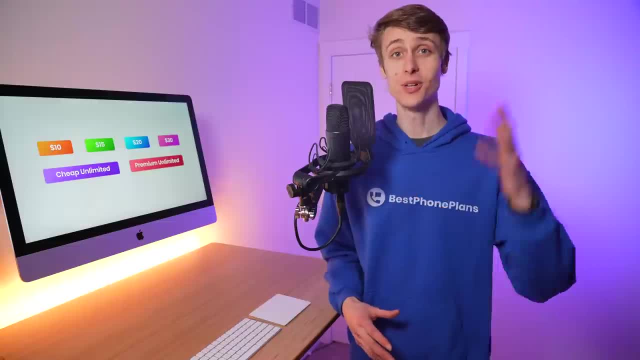 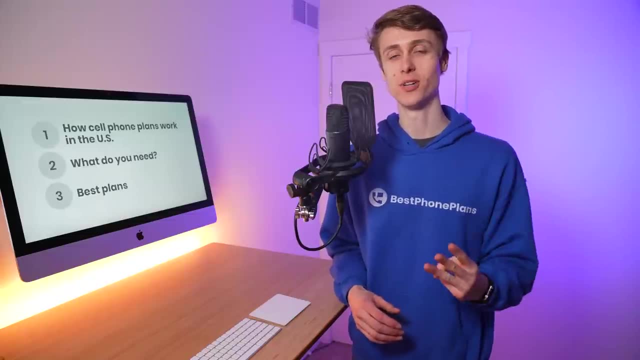 easy for you to find and compare plans. My goal is to help you save money on your cell phone bill, and to do this, we'll be breaking this video down into three main parts: How cell phone plans work in the United States. how to tell exactly how much data you need. 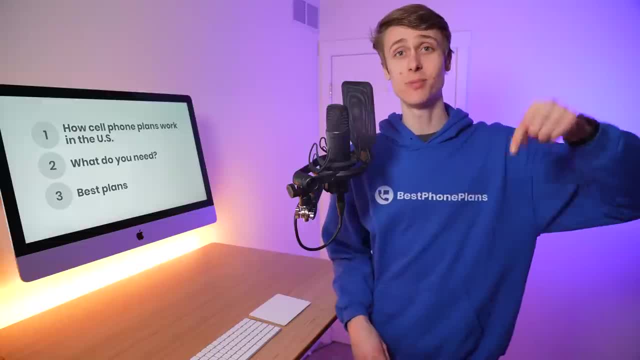 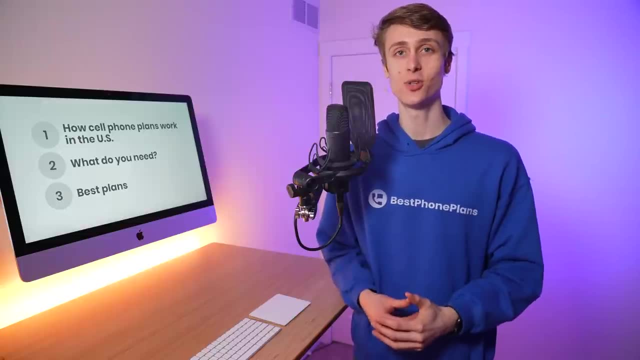 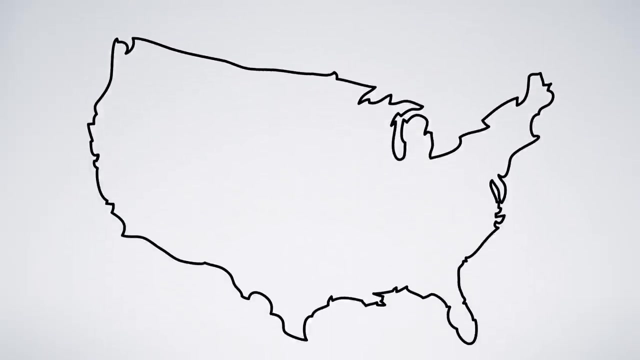 and what the best plans are. Timestamps are linked in the video description so you can jump to the section of the video you're most interested in, and you can find links in the video description to all of the plans and resources we talk about in this video. With that said, let's jump into it. 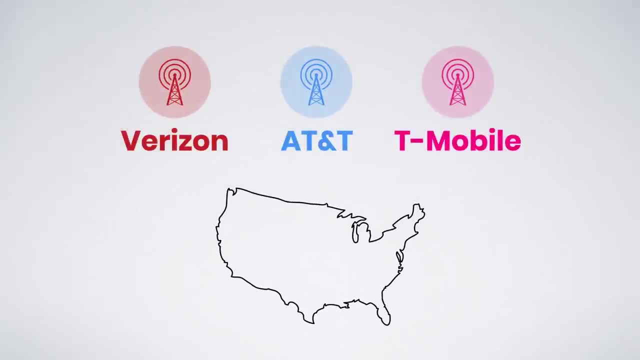 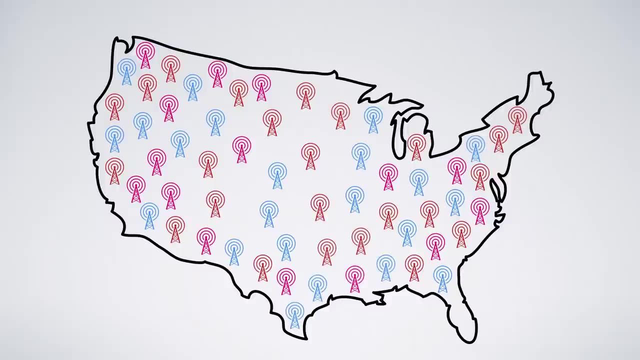 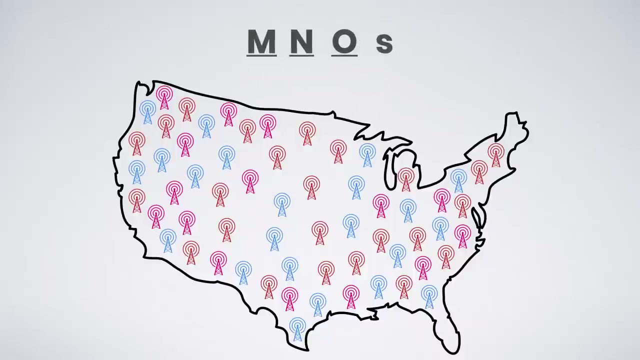 In the United States there are three major carriers: Verizon, AT&T and T-Mobile. These major carriers build cell towers across the United States and operate their own networks. Because they operate their own networks, they are called MNOs or mobile network. 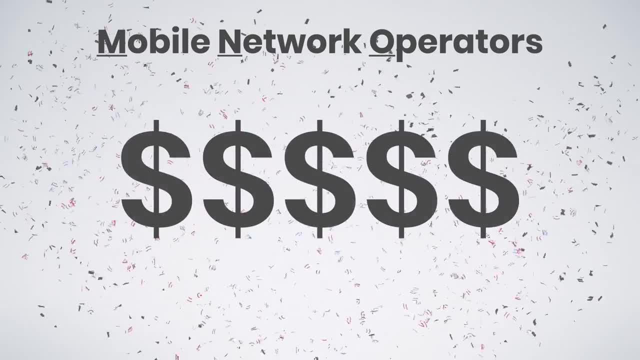 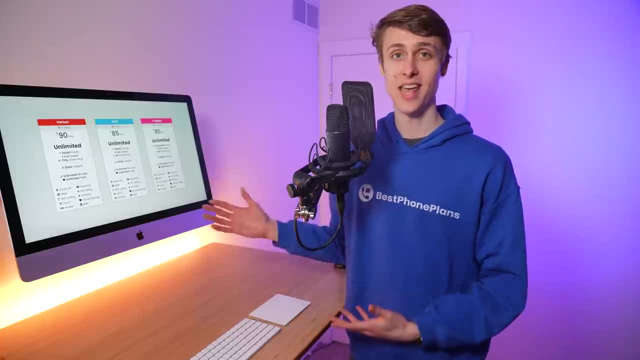 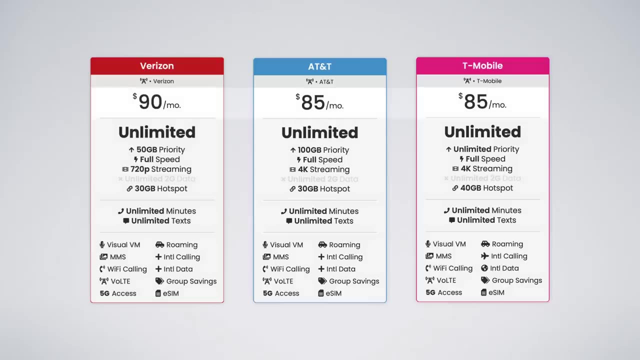 operators. Building a network is expensive, though, so to cover costs, these major carriers charge premium prices for their cell phone plans. These plans can be great for high-income individuals or for families, but the truth is not everyone can afford these $85 to $90 price points. 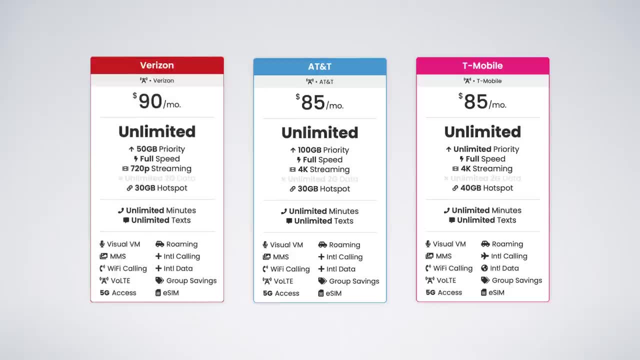 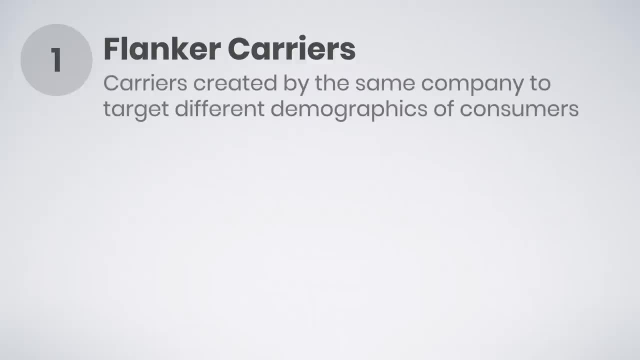 So what do the major network operators do? Well, they do two things. First, they create flanker carriers. Flanker carriers are carriers created by the same company to target different demographics of consumers. Verizon's flanker carrier is visible: for AT&T it's Cricket and on T-Mobile it's the. 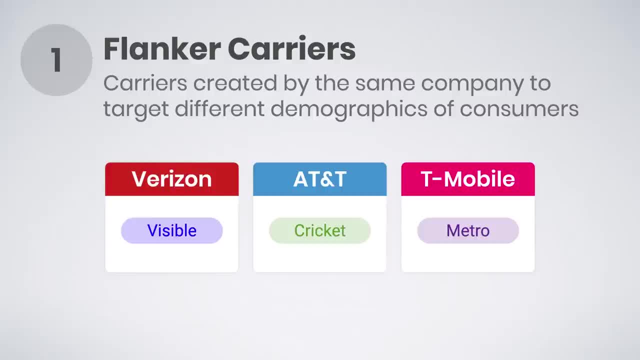 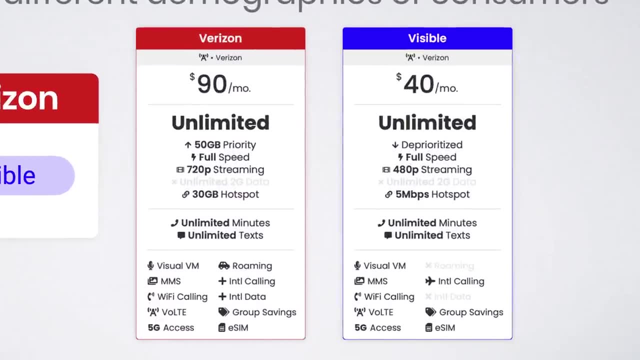 inconspicuously named Metro by T-Mobile. These flanker carriers typically offer significantly more affordable plans. For example, instead of paying $90 per month for an unlimited plan from Verizon, you can pay just $40 per month for an unlimited plan from Visible and save. 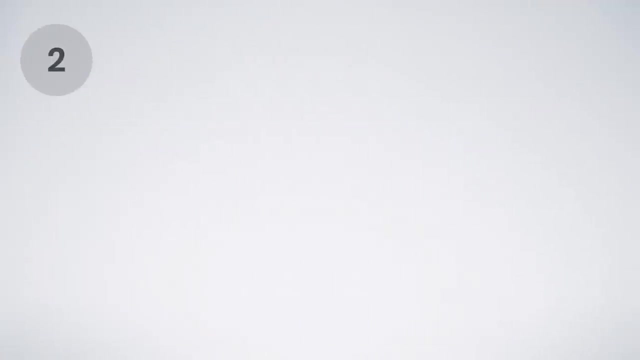 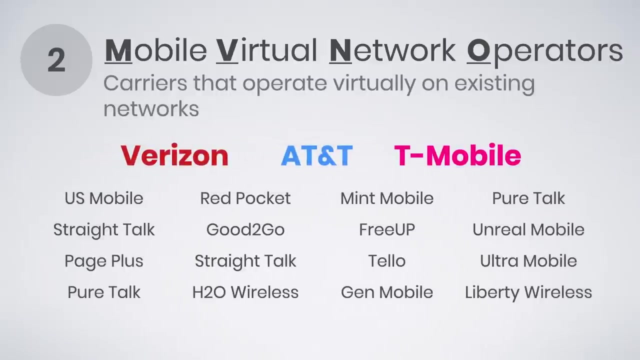 yourself $600 per year. The second strategy the major network operators use is they sell access to their network to MVNOs. MVNO stands for mobile virtual network operator, because these are the smaller carriers operating virtually on the existing networks. Examples include US Mobile, Red, Pocket, Mint, Mobile, Google Play, AirBnB and AT&T, And these sources are 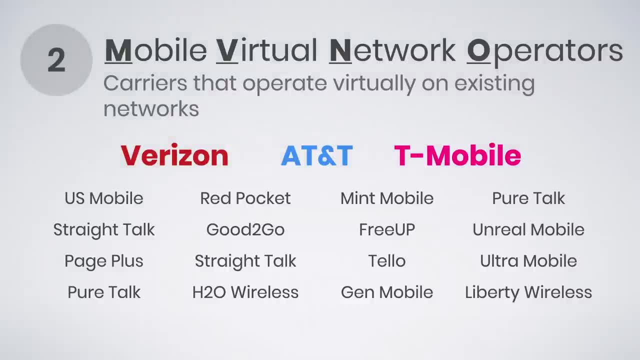 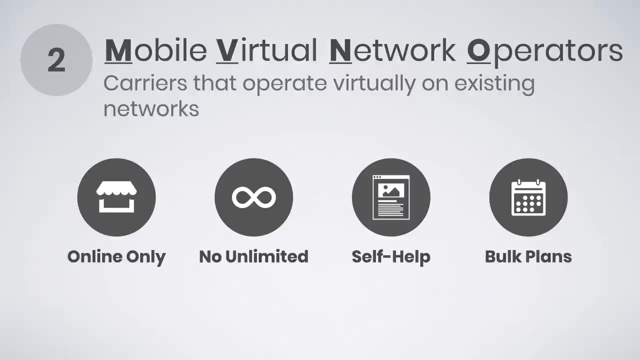 Pure Talk and more. MVNOs are able to offer more affordable plans because they are getting network access at wholesale prices and because they are using cost-saving strategies such as operating online only, not offering true unlimited plans, creating self-help tools. 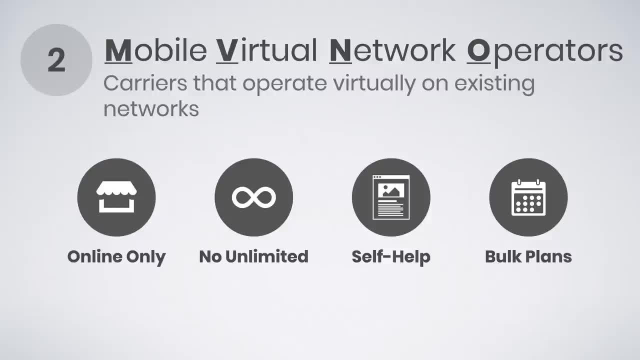 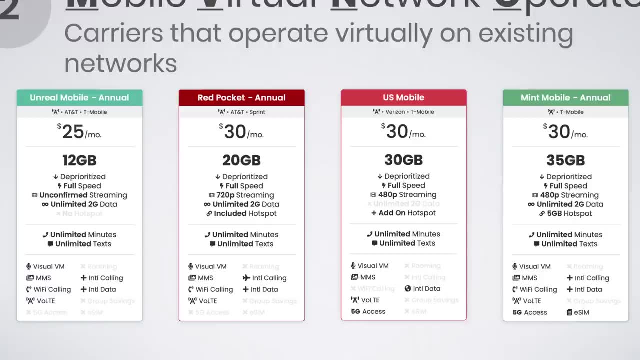 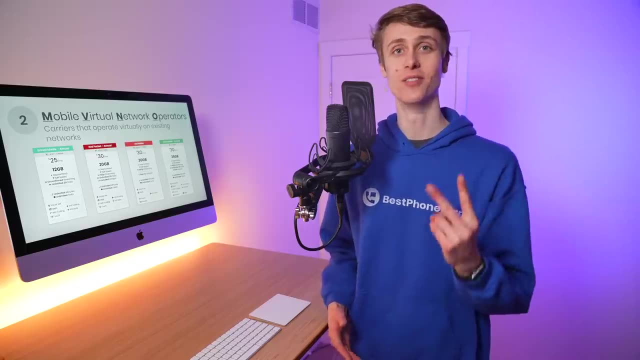 and, more recently, by offering plans in 3,, 6, or 12-month packages. That's how you end up with plans like these, ranging from $25 to $30 per month and including huge amounts of data that go from 12 gigs all the way up to 35 gigs. This brings us to the second part of this video. How much cellular data do you actually need and how do you tell which cell phone plans are right for you? Well, there are four factors to consider when choosing a cell phone plan. First is coverage. You want to get a cell phone plan that you can use at your home. 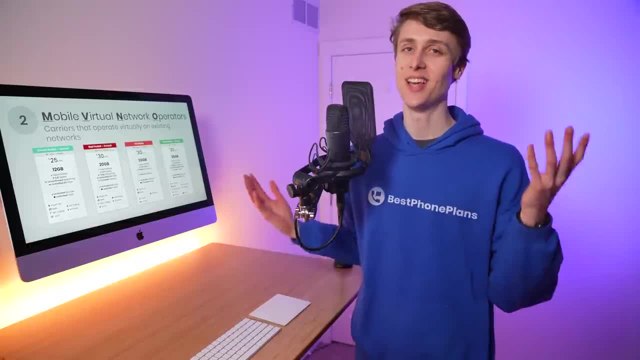 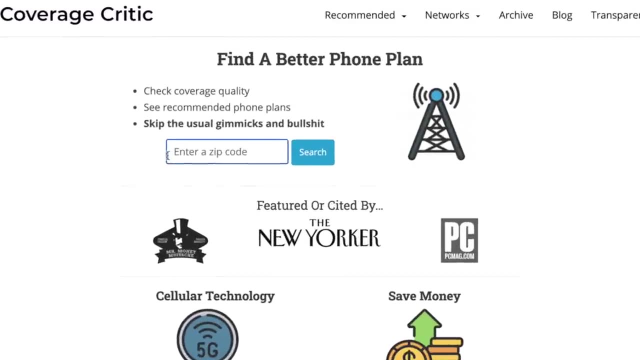 and other locations you frequently visit. If you can't use it, it's not worth having. Thankfully, my friend Chris has built an awesome tool on his site, coveragecriticcom, where you can literally enter your zip code and it'll tell you which network likely has the better performance in your area. 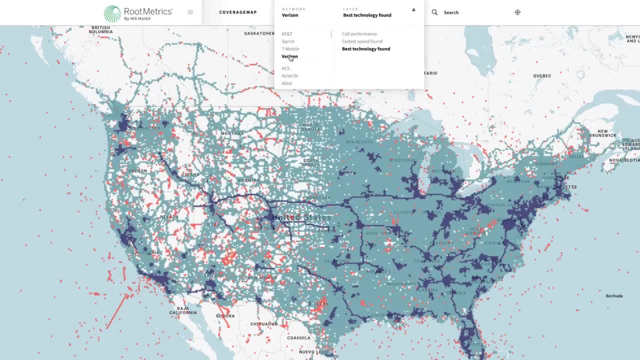 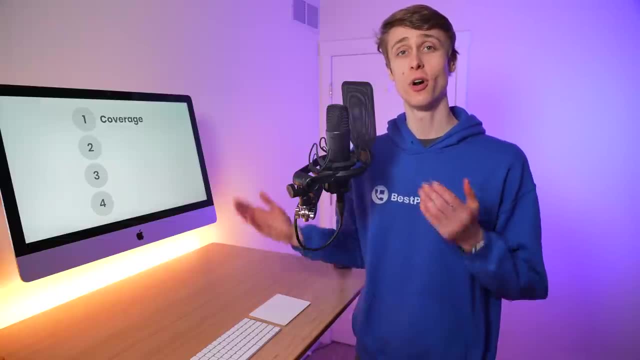 You can also check independent sites like RootMetrics to see coverage and data speeds collected from different users. Or, you know, if you're on the Verizon network right now and it works for you, you can switch to a more affordable plan that also uses the Verizon. 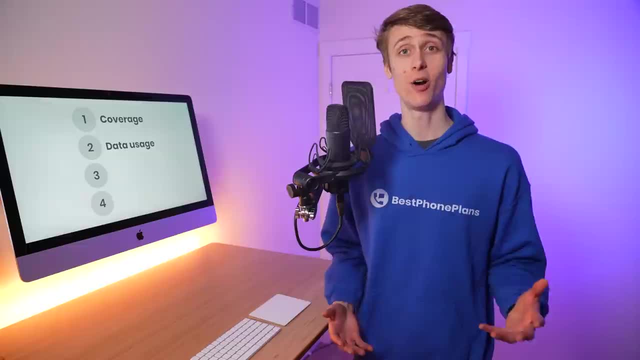 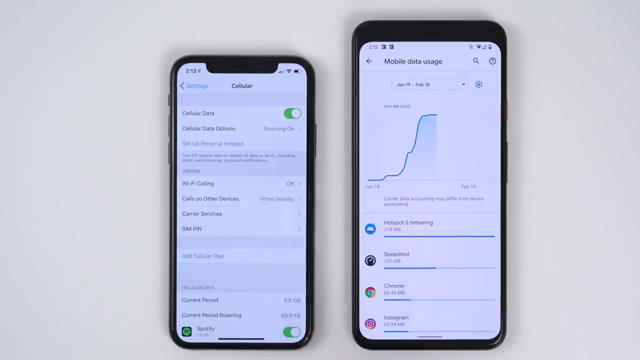 network for coverage. The second factor is data- Data usage. How much data you need plays a big role in which cell phone plans are right for you. Most carriers would like you to believe you need some sort of unlimited plan, but the truth is you likely don't. You can check your actual cell phone data usage in your 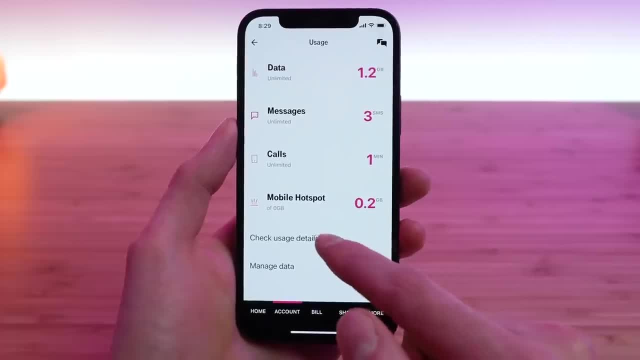 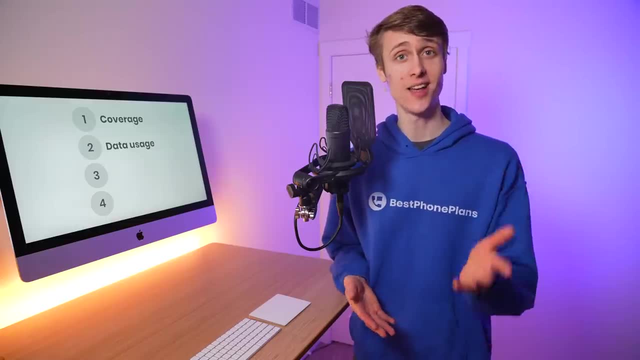 phone settings on iPhone or Android by checking the usage section in your online account or by checking your current bill. Or, if you're like me and lazy, better phrased as time. efficient studies are showing that about 82% of cell phone plans are right for you. 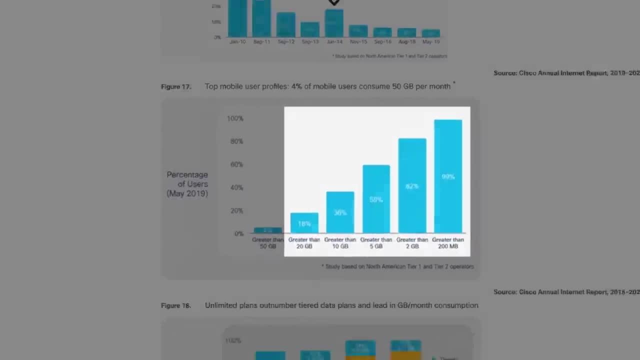 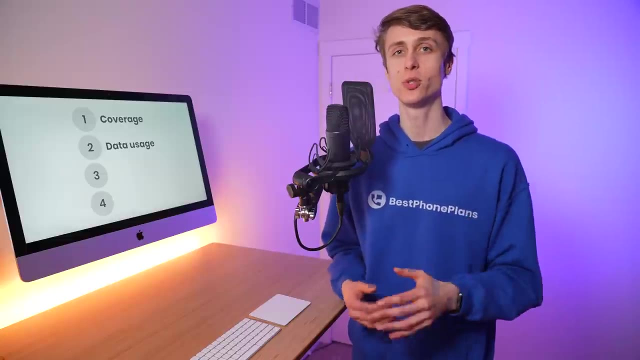 82% of users consume less than 20 gigs of data per month. So odds are that 82% of you watching will be perfectly fine with a cell phone plan that includes about 20 gigs of data. otherwise, in around that $25 to $30 price point. 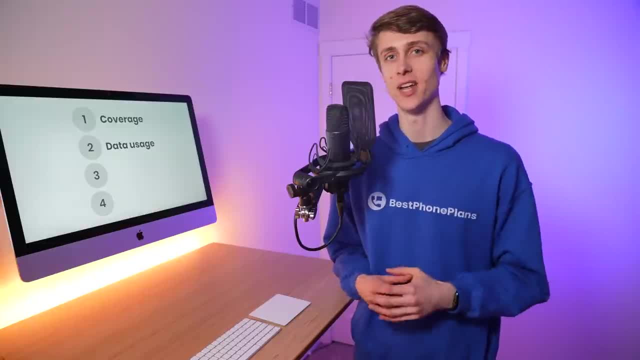 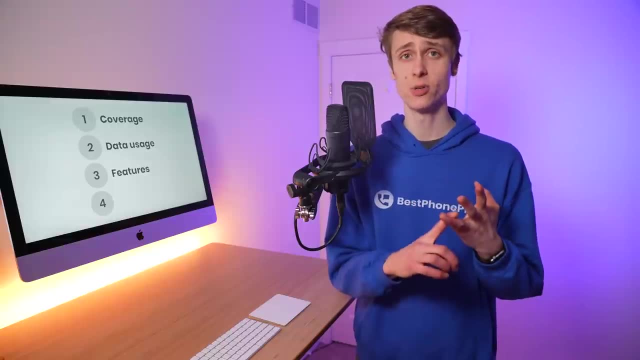 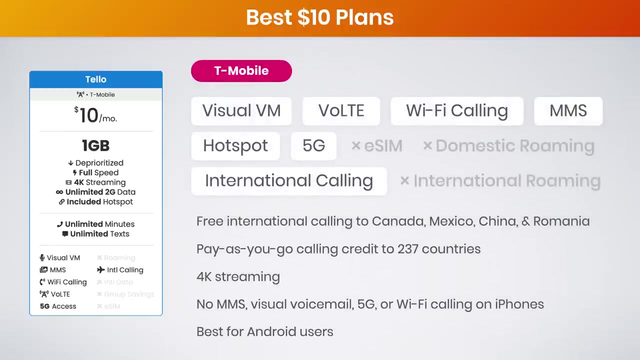 Timestamps are in the video description if you want to jump to that section right now. Third is features. Some people really need features like Wi-Fi calling, eSIM support, international calling, international data roaming or other features. I clearly lay out what features are included with which plan in this video, so if you're 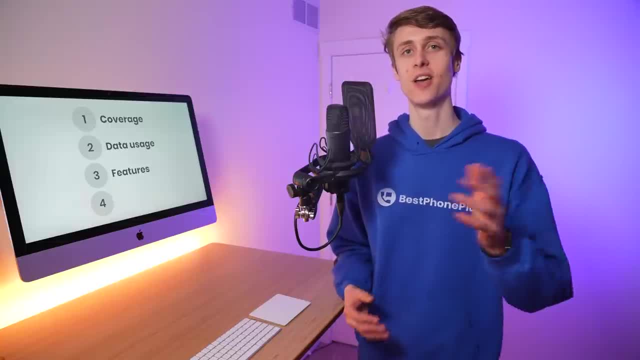 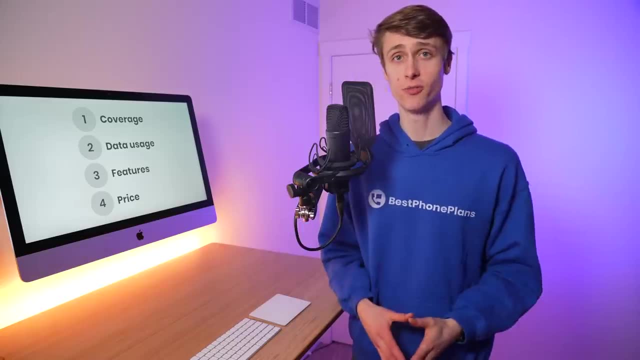 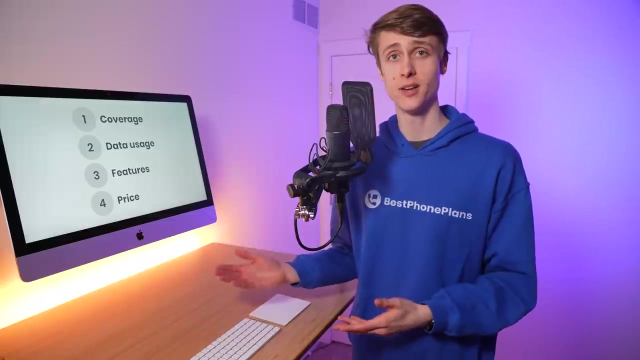 someone who needs a particular feature. just keep your eyes out and I'll make sure you can get a plan that works for you. And fourth is price. How much are you willing to spend on your cell phone plan? Could you curb your usage habits so you use less data and could opt for a more affordable plan? 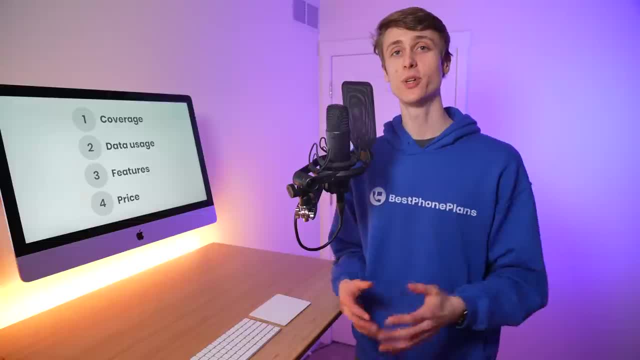 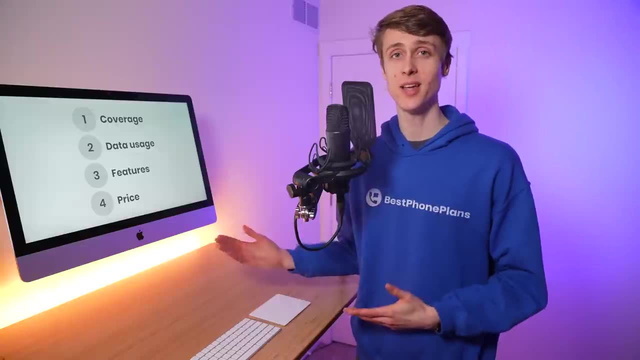 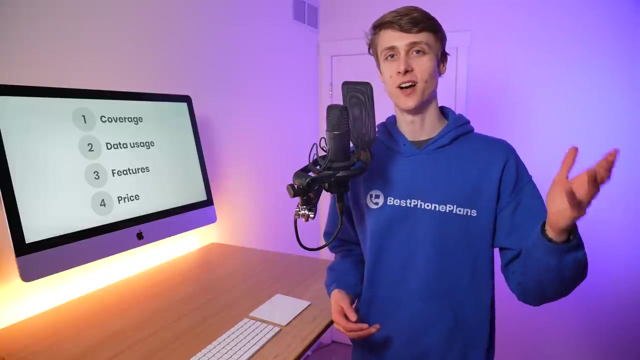 Could you turn on Wi-Fi at home and at work to again reduce your data usage and opt for that cheaper option? Or is it worth it to you to pay for a more premium plan to get extra features and benefits that you need? This is a personal preference, but I'm hoping everyone watching can find an. 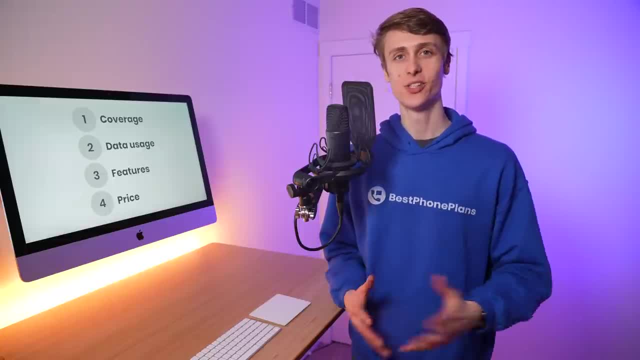 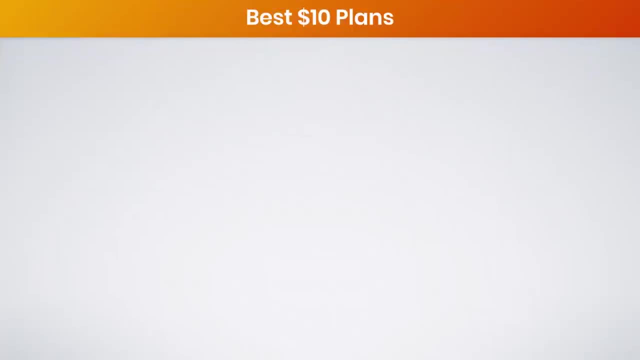 affordable cell phone plan in this video that meets their needs. So, with that said, let's get into the best cell phone plans for 2021.. Starting off, we have the best $10 plans. We have great options here from Tello. 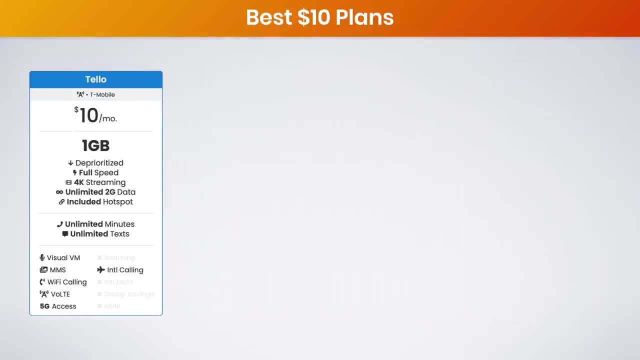 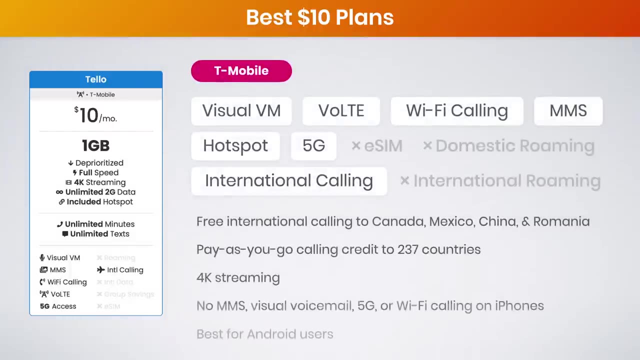 Red Pocket and Unreal Mobile. Let's start with Tello. Red Pocket includes unlimited talk and text with one gig of high-speed data. Tello uses the T-Mobile network for coverage and supports a lot of features, but it turns out many of. 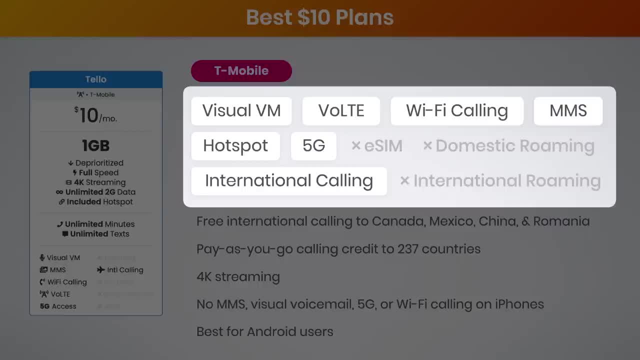 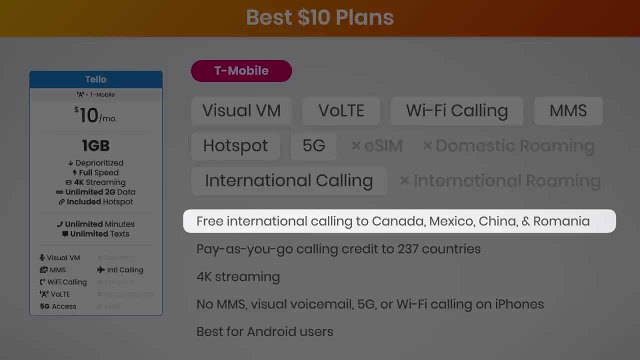 these features are currently exclusive for Android users. MMS, visual voicemail and Wi-Fi calling aren't working on iPhones at the moment. Tello includes free international calling to Canada, Mexico, China and Romania, and you have the option to purchase pay-as-you-go credit to make calls to over 230 other countries. 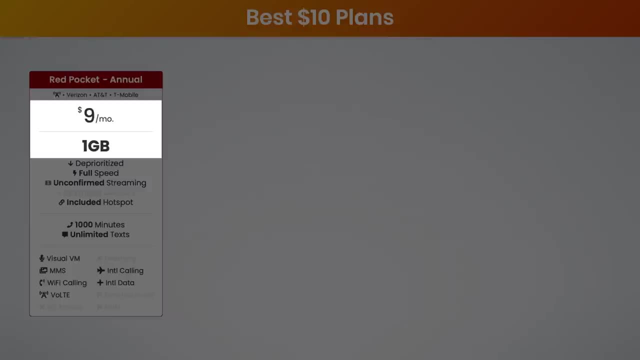 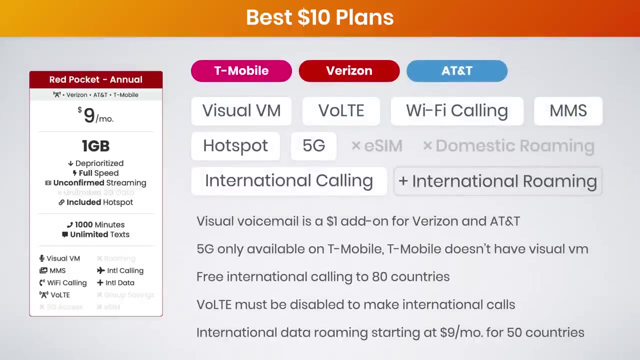 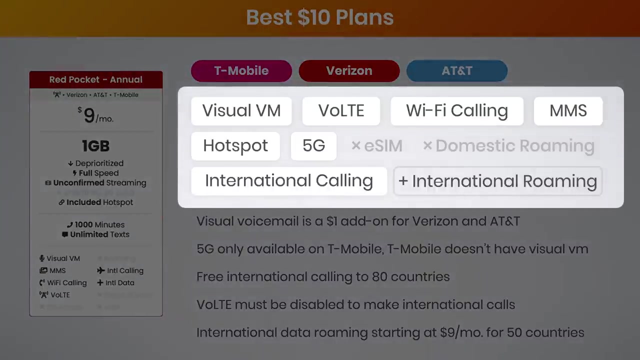 Red Pocket is another great option for you. You can use it to make calls to other countries and it's available on either the Verizon, AT&T or T-Mobile networks. Red Pocket also offers great feature support for both iPhone and Android users. 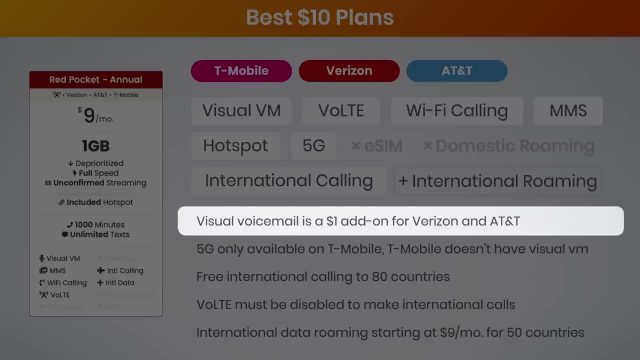 A couple things to note are that visual voicemail is available as a $1 per month add-on for Verizon and AT&T customers, but it's not available for T-Mobile customers, and 5G access is currently only available on the T-Mobile network at the moment. 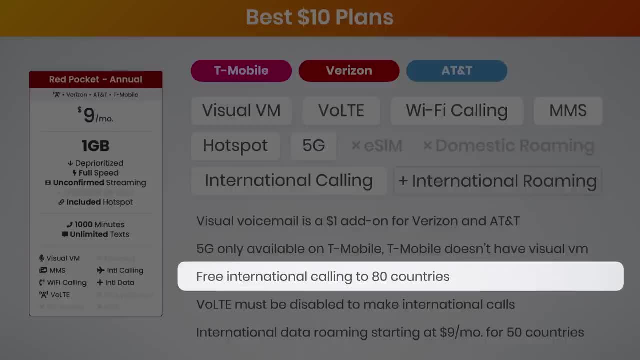 Red Pocket also includes free international calling to 80 countries, though you do have to disable voice over LTE for international calling to work, And they offer an international data roaming add-on starting at just $9 per month for 1GB of data that works across 50 countries. 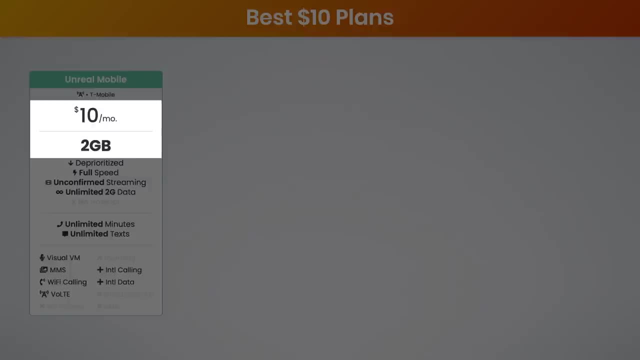 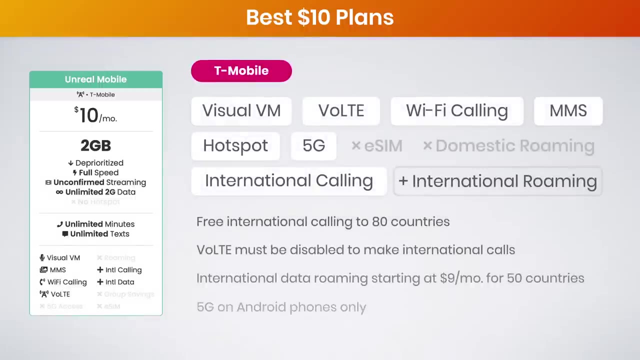 Lastly, in the $10 category, we have Unreal Mobile's $10 2GB plan, and this very well may be the best option here. Unreal Mobile is actually now owned by Red Pocket, so it supports almost the exact same features we saw before. 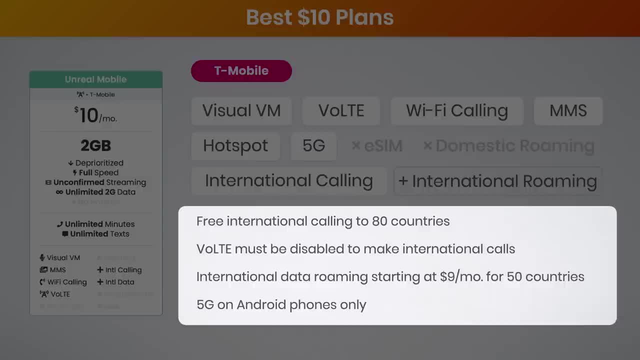 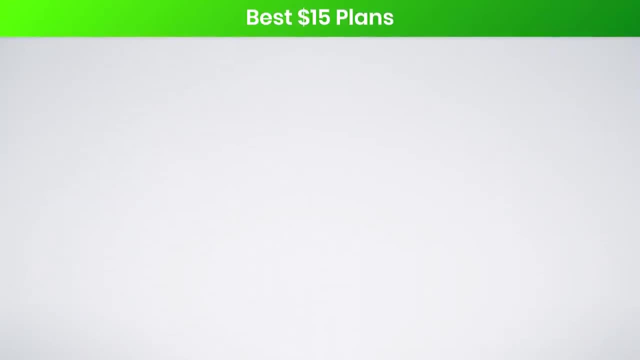 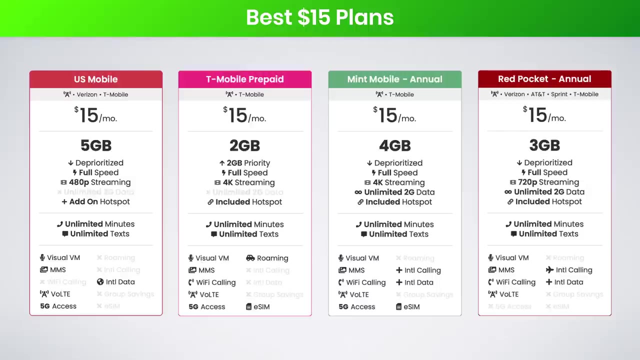 This includes Red Pocket's free international calling to 80 countries, international data roaming add-ons and even 5G access for Android phones. Now let's move on to the best $15 cell phone plans. Here we have fantastic options from US Mobile, T-Mobile, Prepaid, Mint Mobile and Red Pocket. 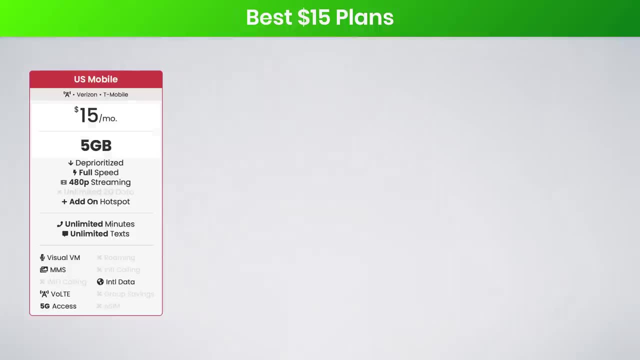 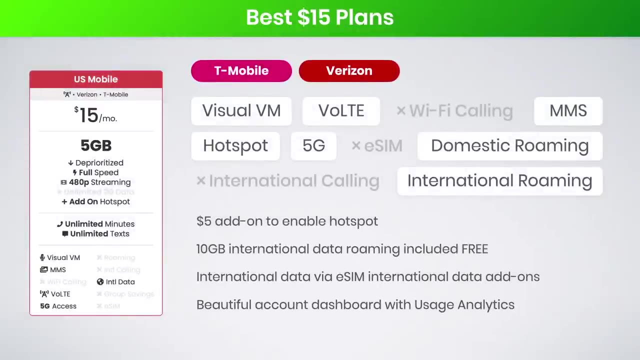 US Mobile's plan is simply one of the best options here. $15 gets you 5GB of data on either the Verizon or T-Mobile network and excellent feature support. You've got voice over LTE, 5G access, domestic roaming on the Verizon network. 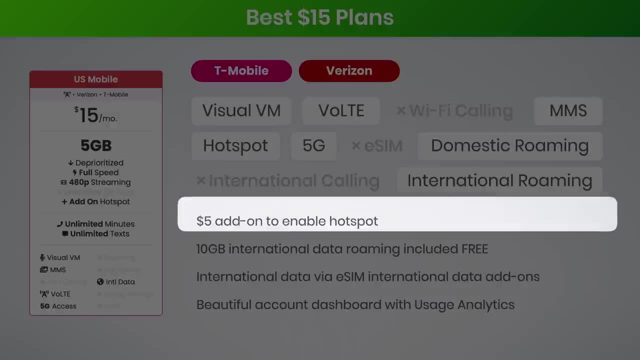 and international roaming all included for free. Hotspot is also available as a $5 add-on. You should also note that the 10GB of international data roaming is included for free, but it's only available as an eSIM data add-on. 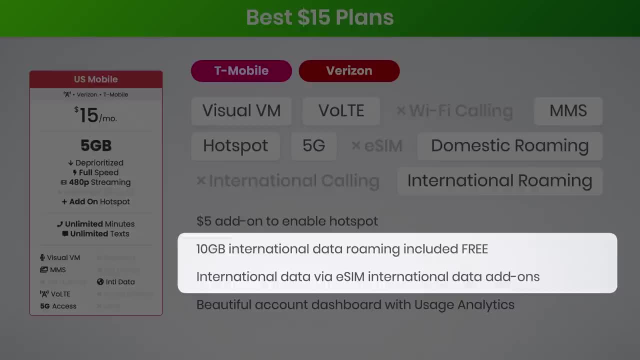 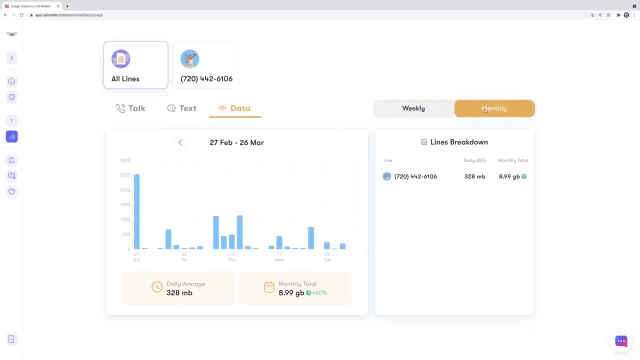 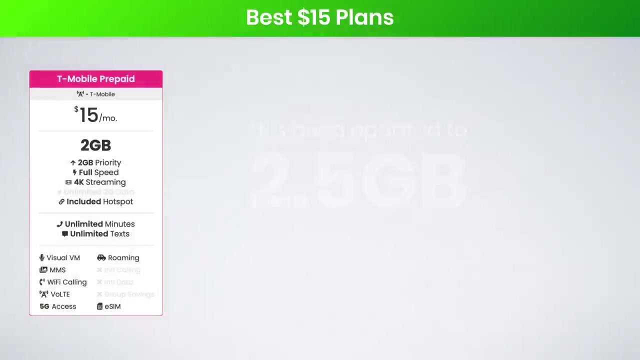 so you'll need to have an eSIM compatible phone to take advantage of this feature. Finally, US Mobile offers a beautiful account dashboard for managing your plans and monitoring your data usage. T-Mobile Prepaid is another decent option here. $15 only gets you 2GB of cellular data. 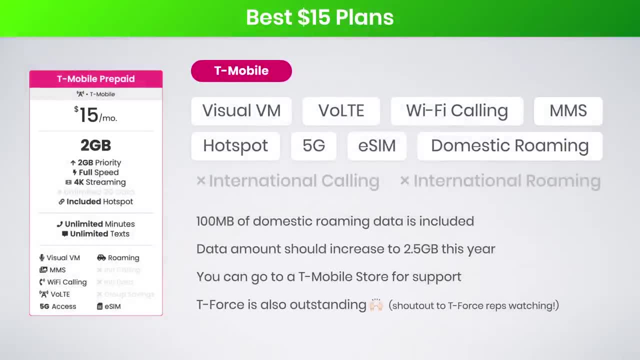 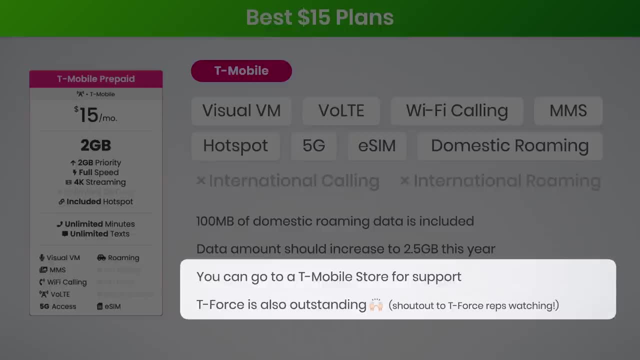 but this plan is packed with features. The notable features are eSIM support, the included 100MB of domestic roaming data and the fact that you can go to a T-Mobile store or contact T-Force for help and support. T-Mobile will also be increasing this plan. 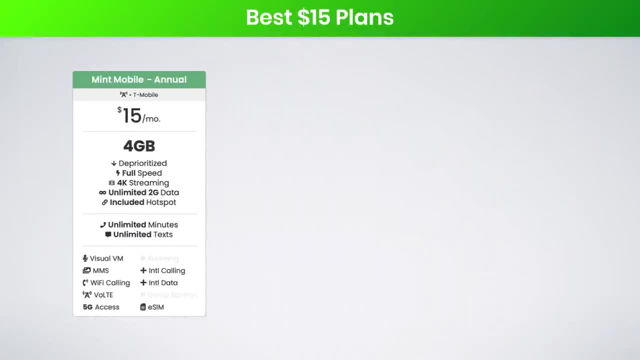 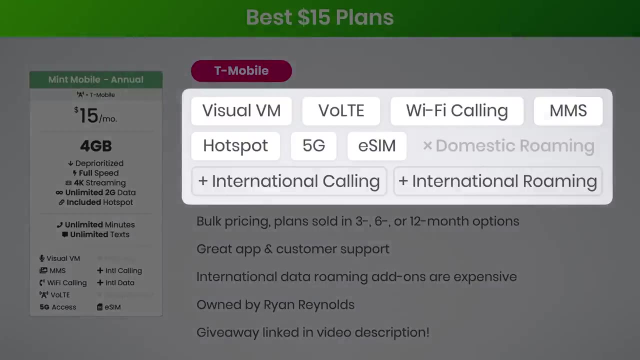 to 2.5GB later this year. Mint Mobile is another carrier that supports a lot of features, including voice over LTE, WiFi calling, Hotspot, 5G access and eSIM, but this time it also delivers an excellent value. 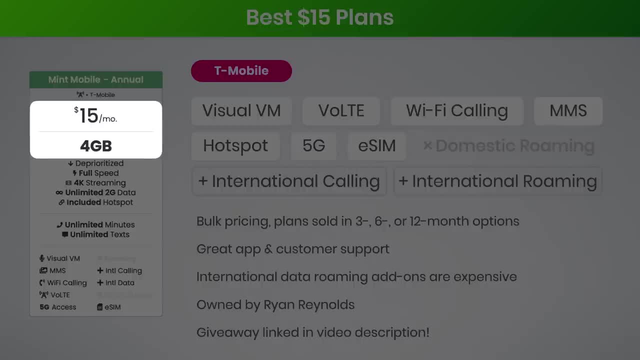 $15 gets you 4GB of data per month- double the amount T-Mobile was offering. Mint is able to offer such a good value because their plans are sold in bulk, either 3,, 6, or 12 month packages. They also offer a great app. and good customer support. Mint Mobile wants to make it as easy as possible for you to try one of their plans, so we are actually partnering together for a giveaway. Each month, Mint Mobile is giving away 1 year of free service on one of their plans. 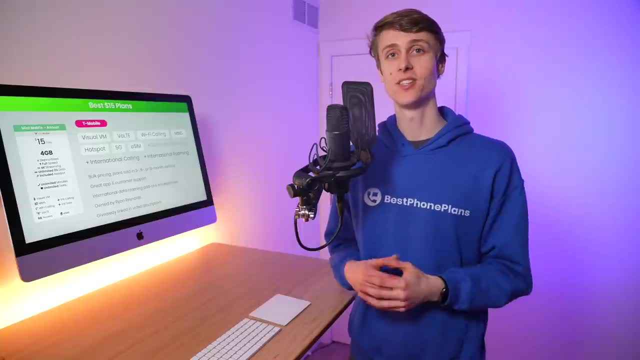 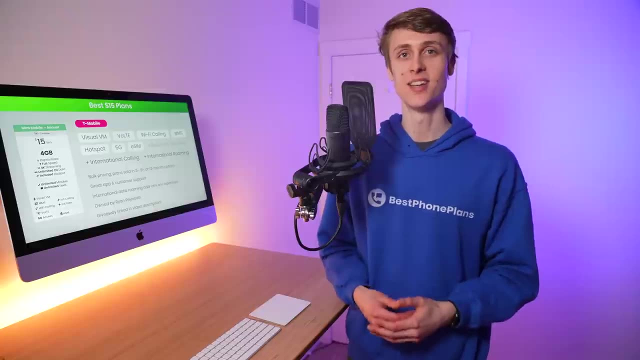 It's currently March, so there are 10 opportunities left to win. A new giveaway will be made available each month, so make sure you come back to this video to enter again. You can enter the giveaway at the link in the video description. 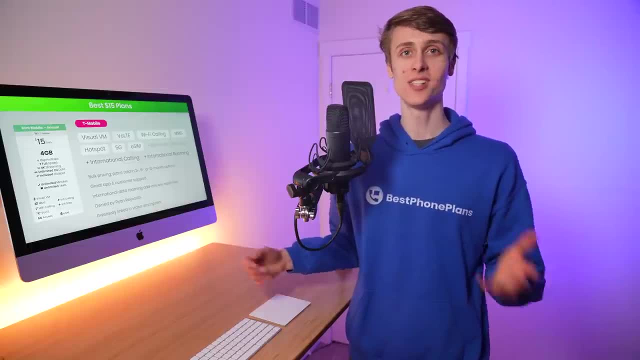 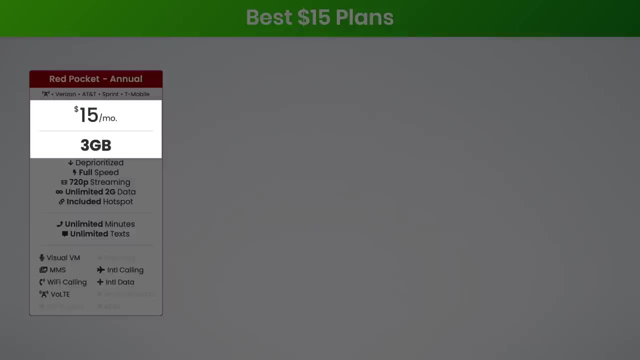 And thank you Mint Mobile for this cool opportunity. I hope one of you wins and enjoys the service. Finally, in the $15 category, we have Red Pocket. This time I'm recommending their $15 3GB plan. This plan continues to support many of the popular features from before. 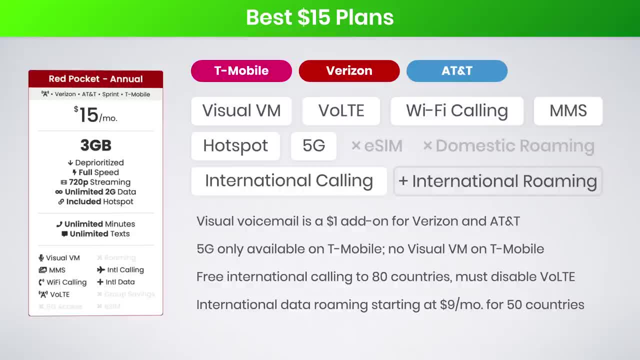 including Red Pocket's international features. I think this plan is best on the AT&T network, because you can find better deals on the T-Mobile and Verizon networks from Mint Mobile and US Mobile. Next, we have the best for you: Mint Mobile. 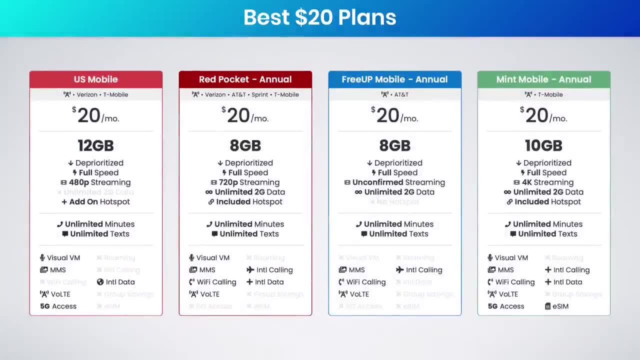 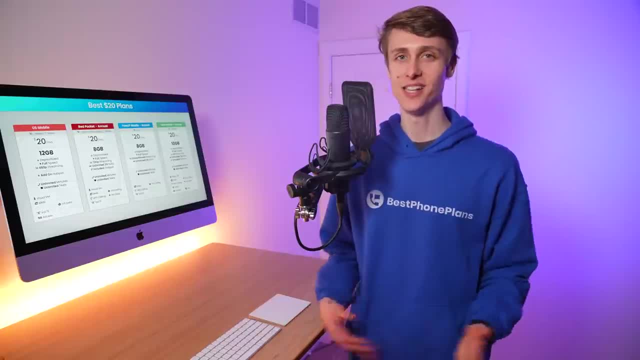 What you'll see are full features that you can't afford to buy $20 plans. We have great options here from US Mobile, Red Pocket, FreeUp Mobile and Mint Mobile, And if you're enjoying the video so far, please give it a thumbs up down below, as I would. 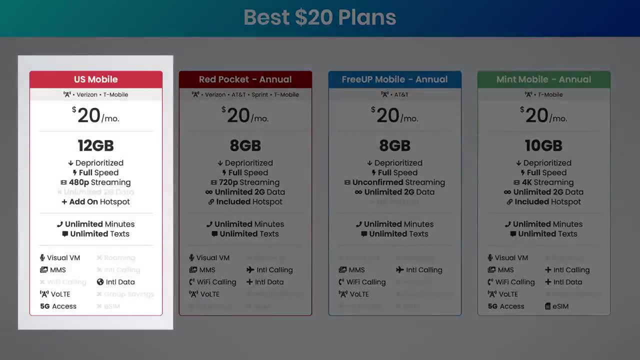 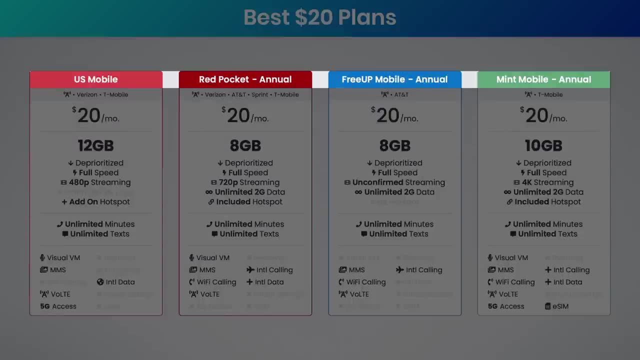 super, appreciate it. US Mobile's $20 12 gig plan is probably one of my favorite options here. It not only includes the most data, but it's also a monthly plan as opposed to an annual plan. US Mobile's plan is available on Verizon or T-Mobile and it includes the same features. 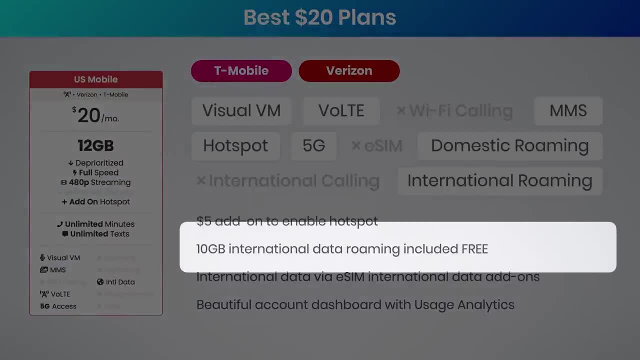 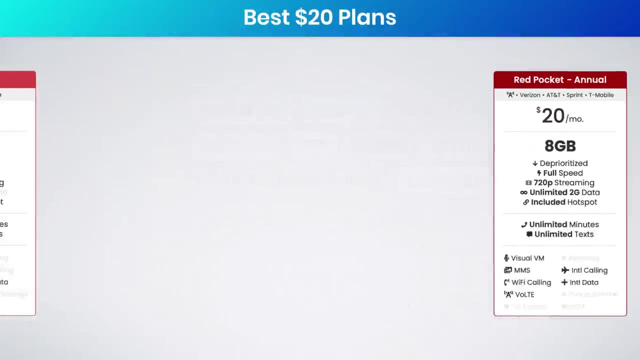 we've talked about before. Hotspot is still $5 to enable and you're still getting the 10 gigs of international data roaming included for free via the international eSIM add-on. Next up, we have another plan from Red Pocket. Their $20 plan includes 8 gigs of high-speed data. 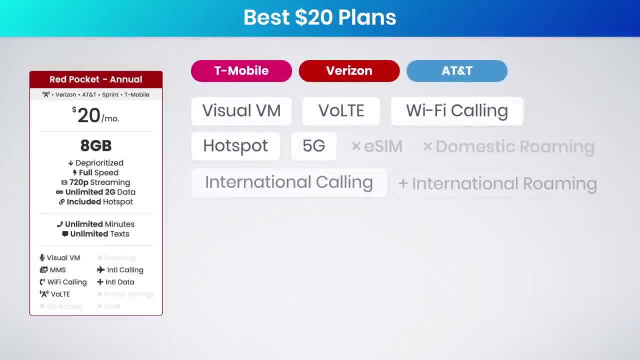 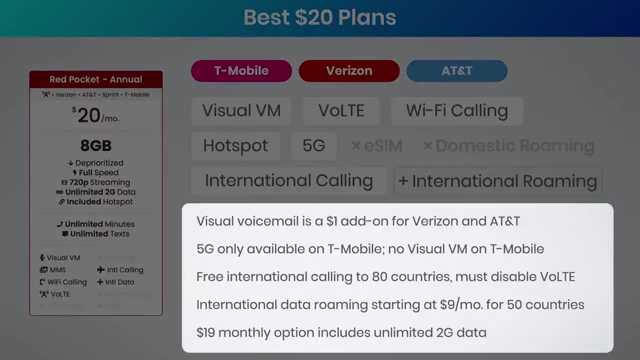 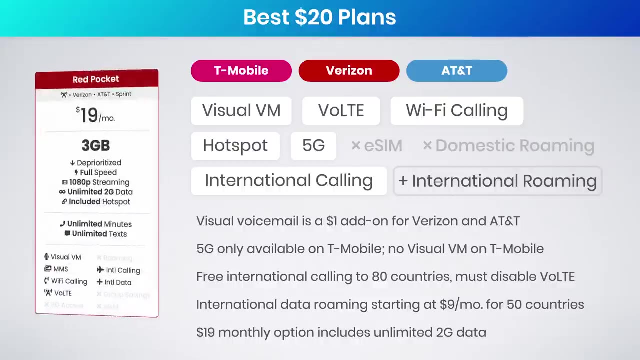 before unlimited data at 2G speeds. This plan is available on the Verizon, AT&T or T-Mobile networks and it includes decent feature support, along with Red Pocket's excellent international calling perks and international data roaming. If you'd prefer to pay monthly, Red Pocket does offer a $19 plan. 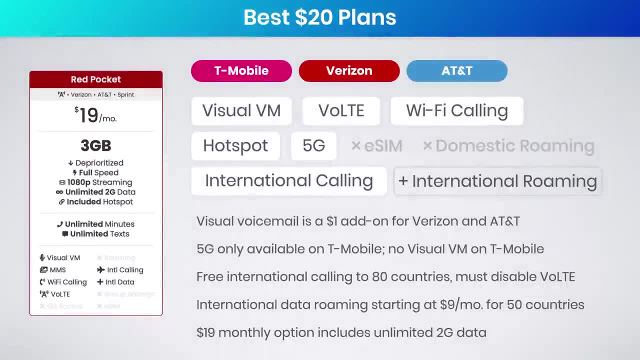 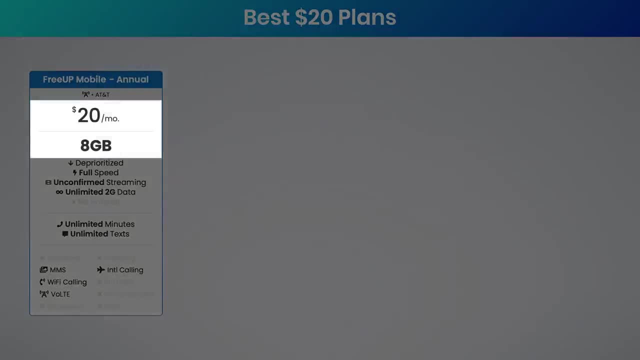 but the data amount drops from 8 gigs down to only 3 gigs. FreeUp Mobile's plan is another option to consider. on the AT&T network, They similarly offer an annual plan that breaks down to $20 a month and includes 8 gigs of high-speed data. 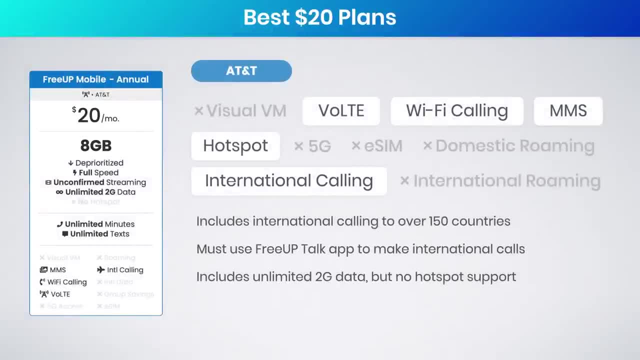 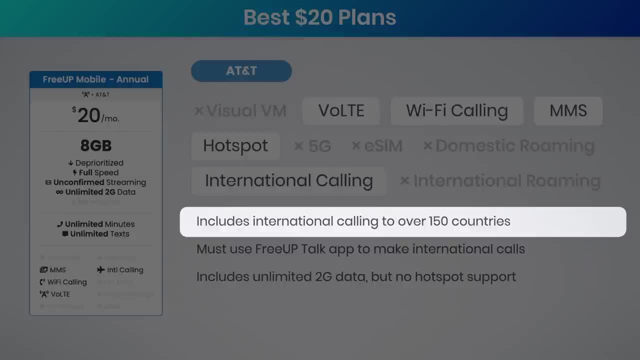 FreeUp Mobile is missing support for visual voicemail- but it actually includes even better international calling than Red Pocket. You can make calls to over 150 companies, and you can also make calls to over 150 companies. Lastly, in this category we have the plan that I use personally for my primary phone. number. It's Mint Mobile's $20 plan with 10 gigs of high-speed data. What I love about Mint is they support all of my favorite features, including Wi-Fi calling, hotspot 5G access and even eSIM, and I feel their plans are a tremendous value. Oh, and a friendly reminder: 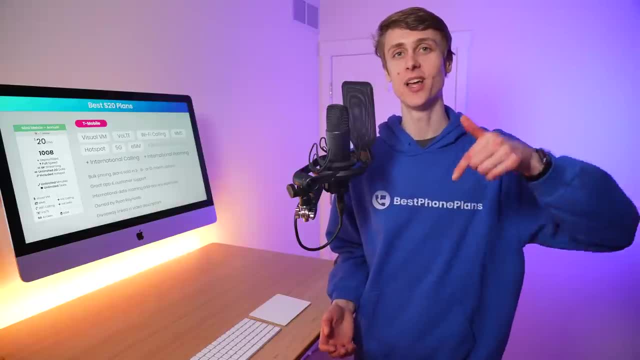 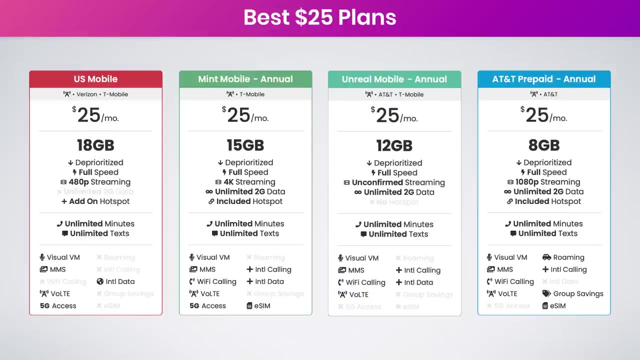 you can win a year of free Mint Mobile service at the giveaway linked in the video description. Now let's get into the plan. Now let's move on to the best $25 plans And, honestly, these may be some of the best value. 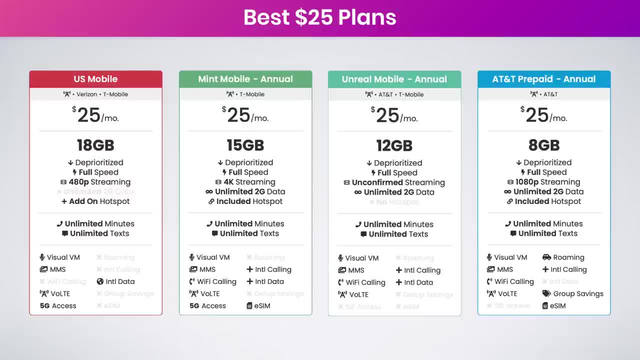 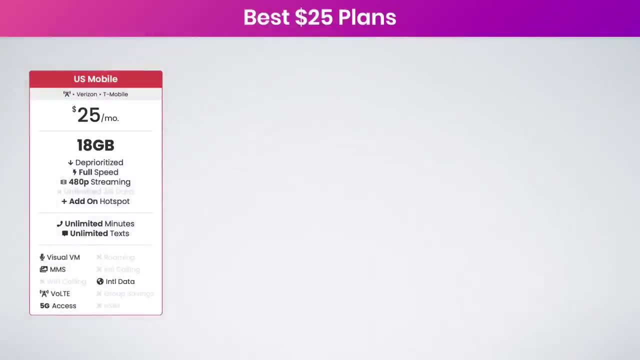 plans out there, perfect for average users and individuals. First up is US Mobile's $25 18-gig plan. This includes a huge amount of data at an affordable price and it continues to support the features US Mobile is known for. Their most notable features are their impressive. 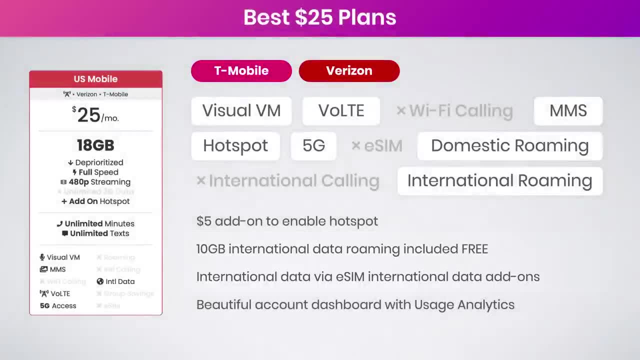 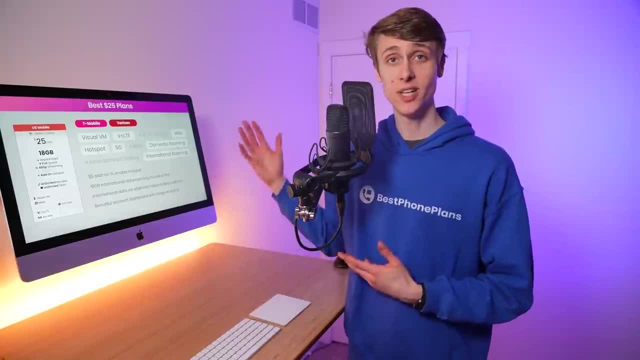 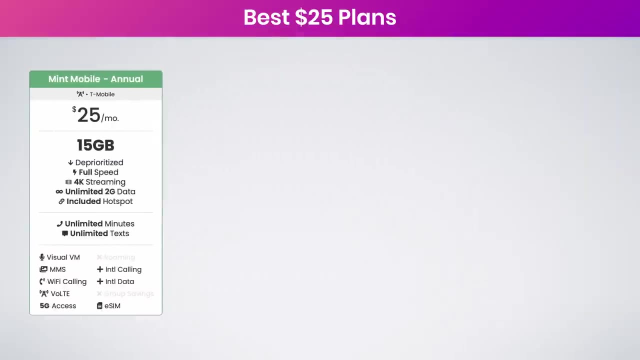 10 gigs of international data available via eSIM and their beautiful online account dashboard with detailed usage analytics to manage your account. This is also the only monthly plan here, giving you the flexibility to switch plans anytime you want. Next we have Mint Mobile's $25 15-gig. 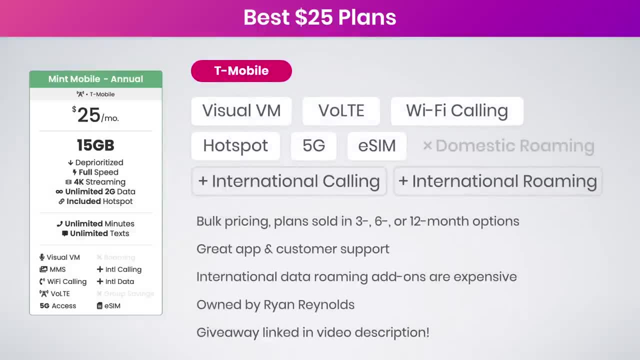 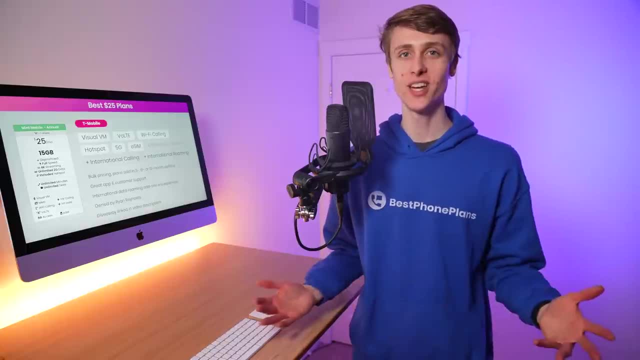 plan Similar to before. I love Mint Mobile for their excellent feature support, great application and good customer service. Mint Mobile's giveaway is linked in the video description if you'd like a chance to win a year of free service, And the reason I keep mentioning it is because I'm 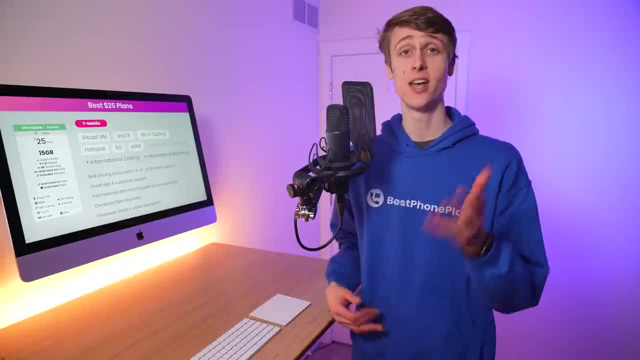 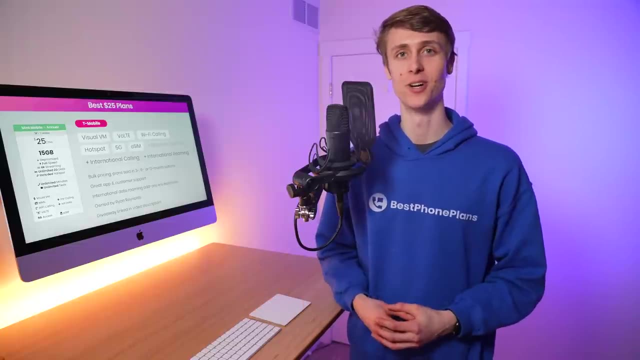 imagining some of you are still watching this video. So if you're interested in getting a chance to win a year of free service, make sure you subscribe to my YouTube channel and hit the bell icon so you don't miss out on any of the new videos I upload. 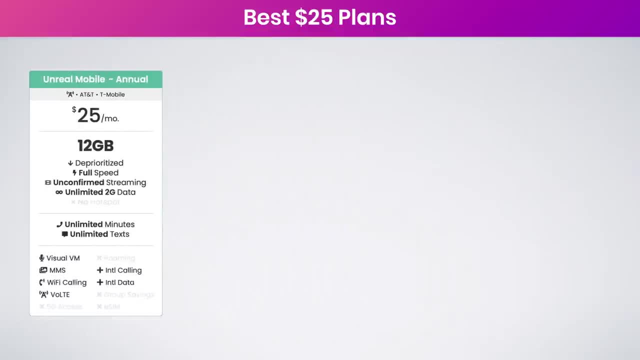 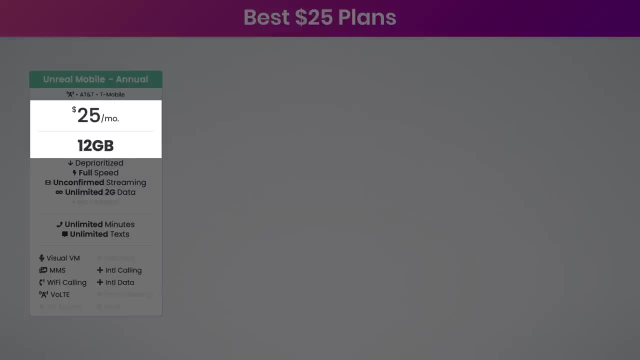 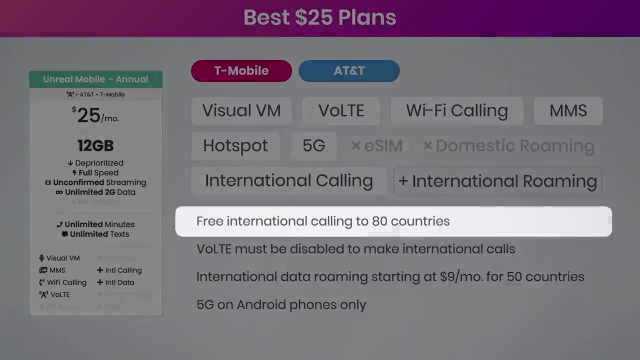 Unreal Mobile is another competitive plan in this category and they offer some of the most data you can get on the AT&T network. $25 for 12 gigs is an excellent value. Unfortunately, no hotspot support here, but as Unreal Mobile is owned by Red Pocket, you do get international calling. 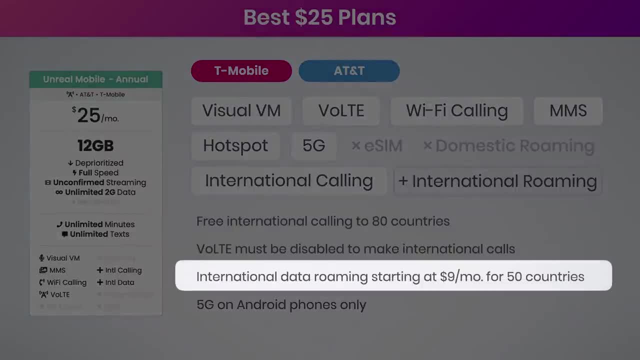 included for free, and the opportunity to win a year of free service is great. So if you're interested in getting a chance to win a year of free service, make sure you subscribe to my YouTube channel and hit the bell icon so you don't miss out on any of the new videos I upload. 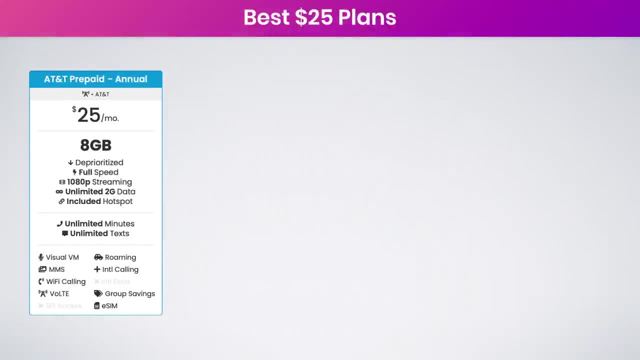 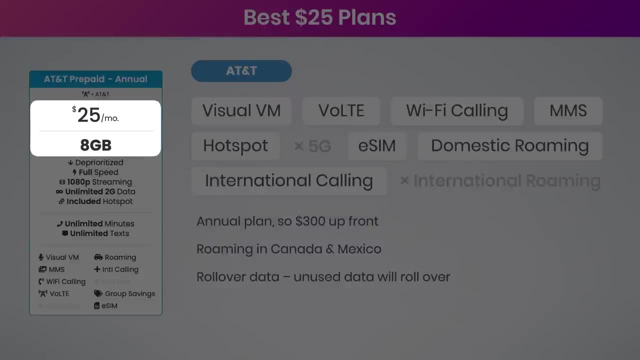 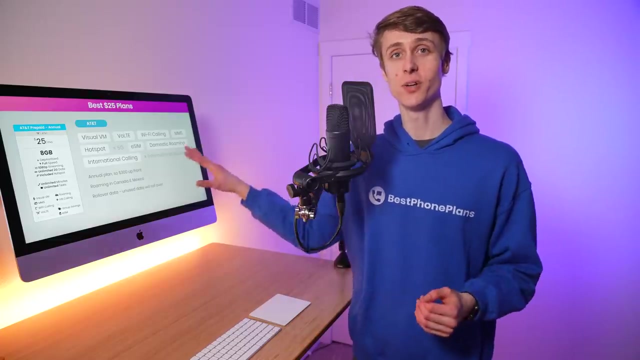 Lastly in this category, we have a plan from AT&T themselves, and it's their annual prepaid plan. This plan is $300 up front, but it breaks down to just $25 per month and includes a decent 8 gigs of high-speed data. Many viewers actually voted. this was one of the best plans on the AT&T. 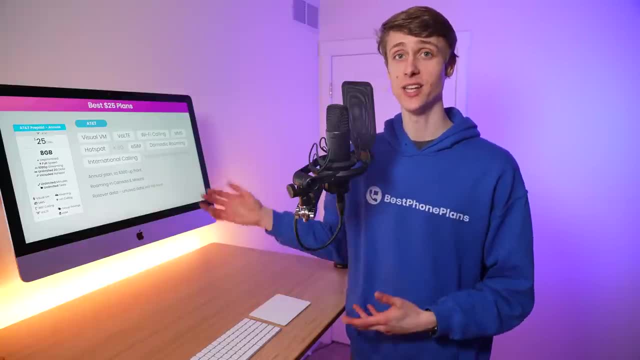 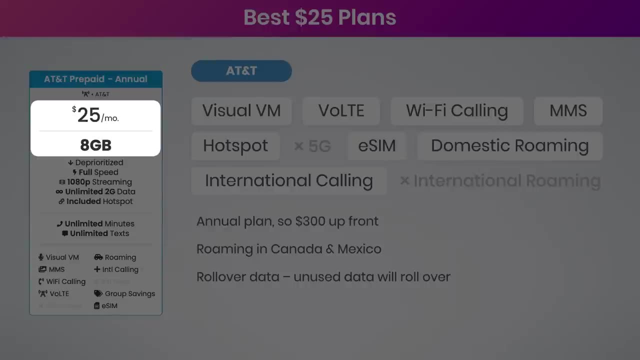 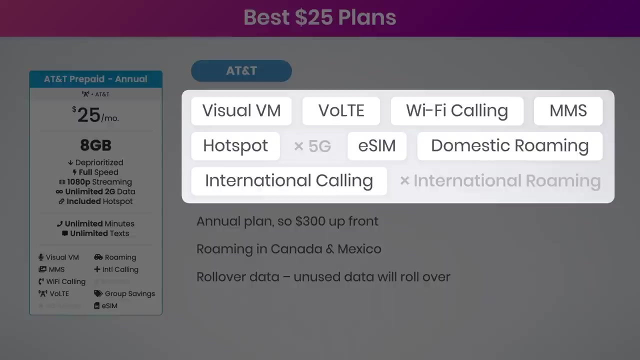 network at this price point because of the features it supports. It may not be as good of a value as Unreal Mobile, which offered 12 gigs compared to AT&T's 8 gigs, but by going with a plan from AT&T directly you get excellent feature support. Notable features include Wi-Fi calling, eSIM. 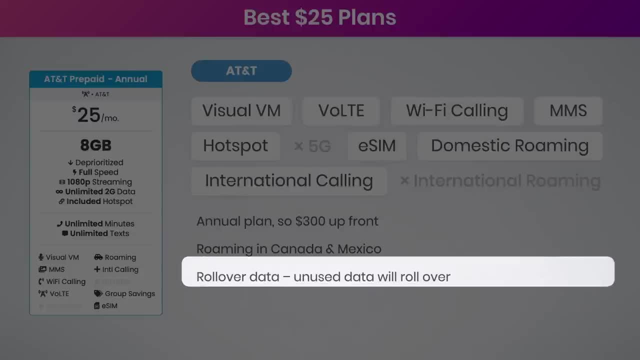 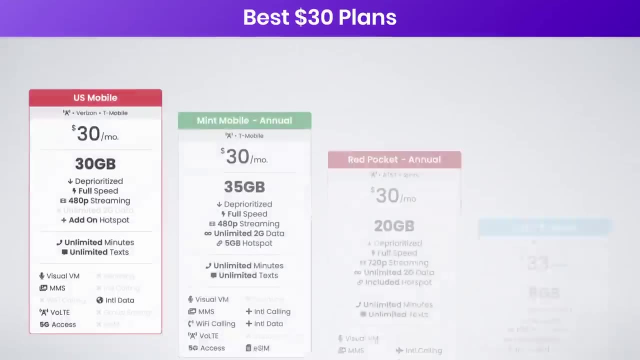 domestic roaming, roaming in Canada and Mexico- and rollover data, So unused data will rollover each month. Now we have the best $30 plans. Like the $25 plans, these continue to be some of the best value plans in the industry. They offer enough data to be able to run a lot of work. 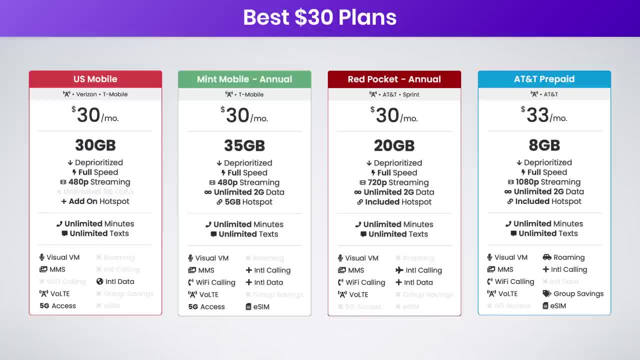 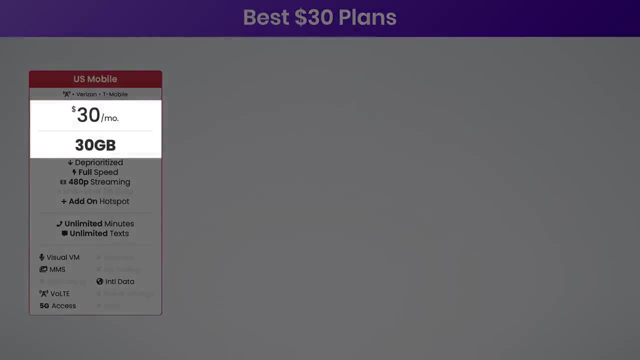 for over 82% of average consumers at incredibly affordable prices. US Mobile continues to be one of my favorite options. Their $30 plan includes 30 gigabytes of high-speed data and is available on Verizon or T-Mobile. Notable features include 5G access. 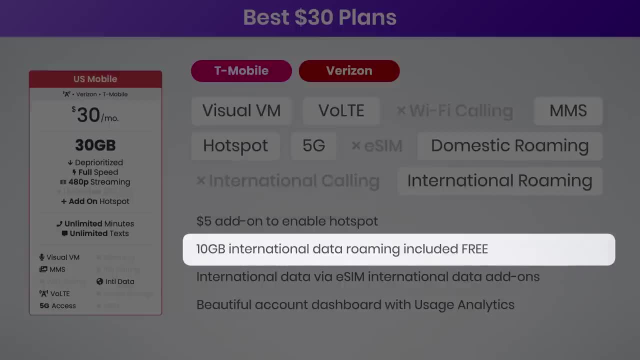 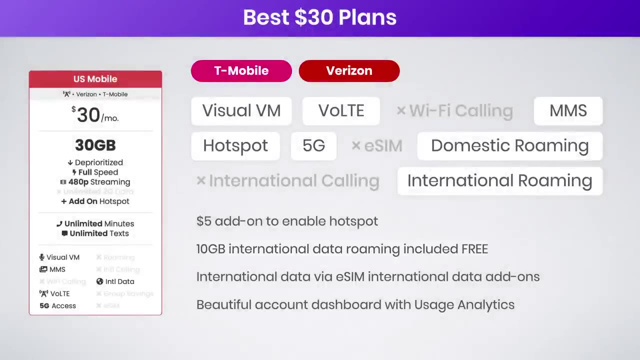 on both Verizon and T-Mobile, and the included 10 gigs of international roaming data available via the international eSIM add-ons. What's also powerful about this plan is, with US Mobile's usage analytics, it's able to run a lot of work in a few days. So if you're looking for a 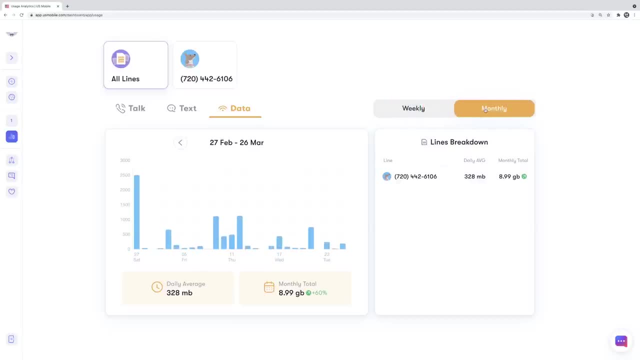 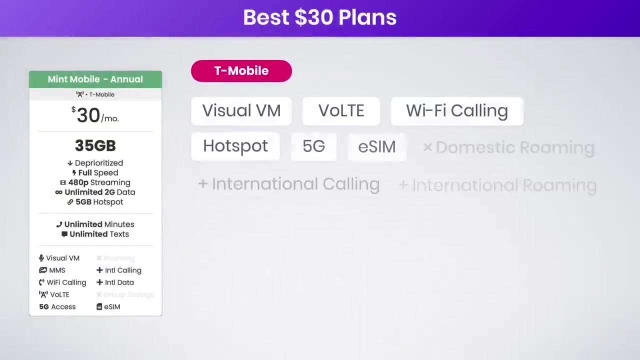 dashboard, you can know exactly how much data you're using And if it turns out you need less data, you can switch to one of US Mobile's more affordable plans and save yourself even more money each month. Next in this category, we have Mint Mobile's $30- 35 gig plan. This offers excellent. 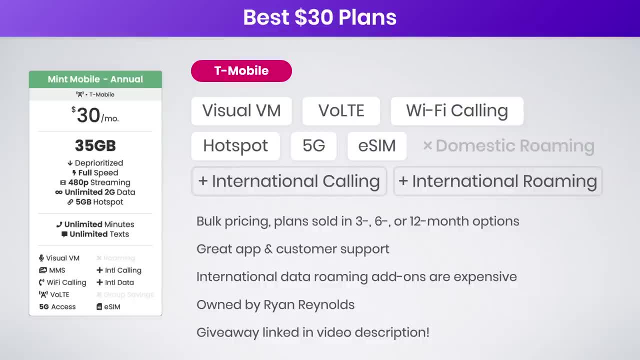 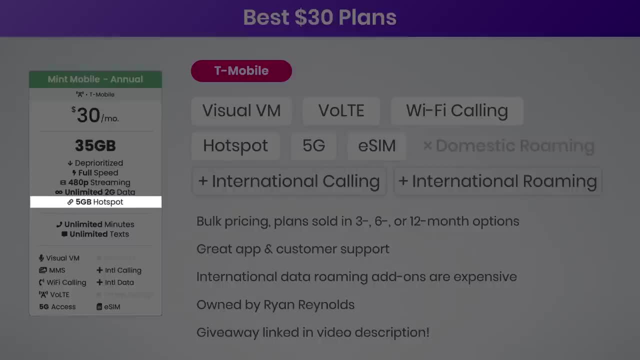 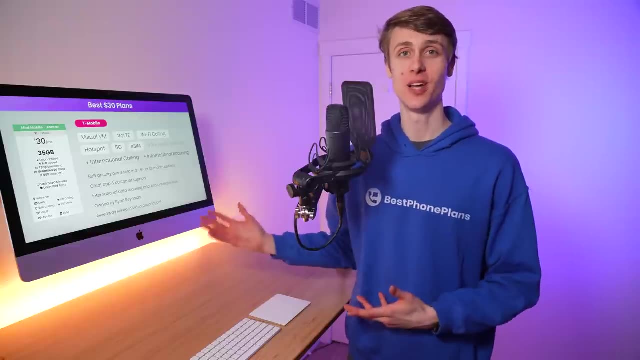 feature support like all of Mint Mobile's other plans, but there are two key differences: Video streaming is limited to 480p instead of 4K and you only get 5 gigs of high-speed hotspot data instead of being able to use all of your included data as hotspot data. I still love this plan. 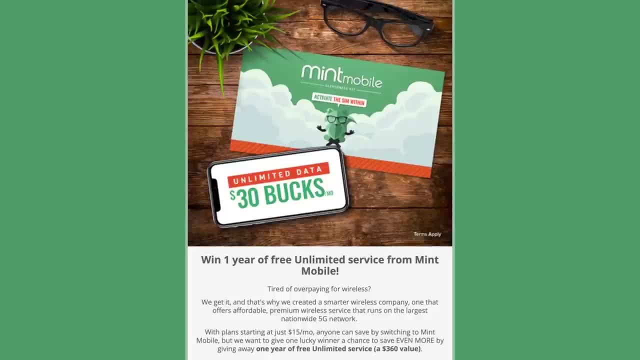 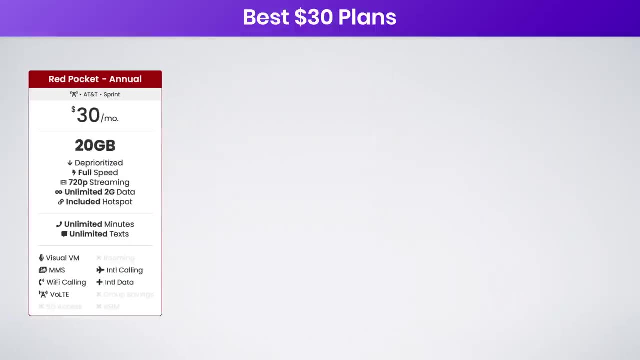 though, and this is actually the plan Mint Mobile is giving away right now, in March, at the giveaway linked in the video description. Finally, we have two plans on the AT&T network rounding off this category. The first is Red Pocket's annual plan offering 20 gigs of data for $30 per month- Red. 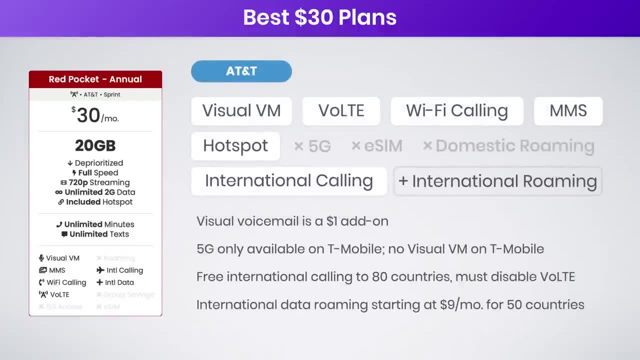 Pocket continues to be a great option for anyone looking for a plan that includes international calling and affordable internet access. The second is Red Pocket's annual plan offering 20 gigs of international data roaming add-ons. If you'd prefer to pay monthly, Red Pocket also offers. 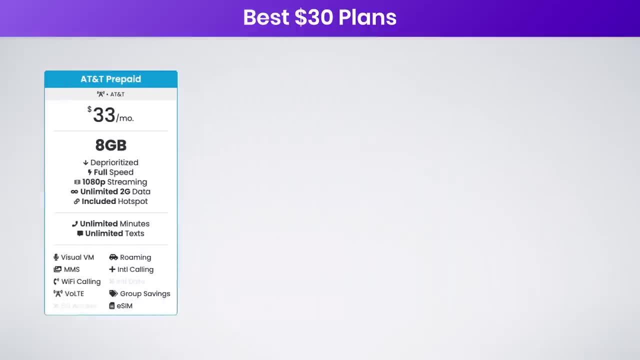 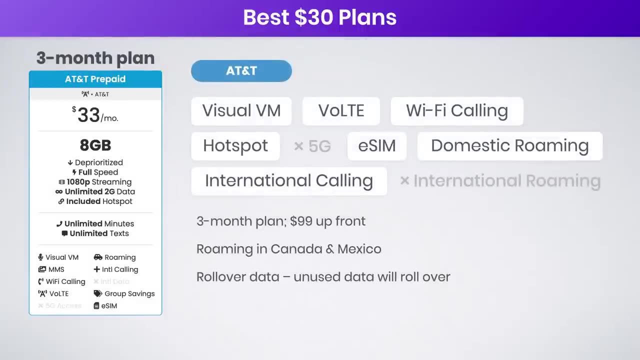 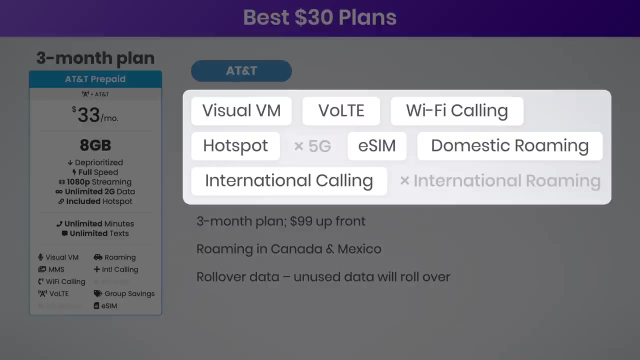 a $30 10 gig plan. And the second great option on the AT&T network is AT&T's $33 prepaid plan. This is actually a three-month plan, so $99 up front. It doesn't include nearly as much data as Red Pocket but again, what people liked about this plan is the feature support: You get Wi-Fi. 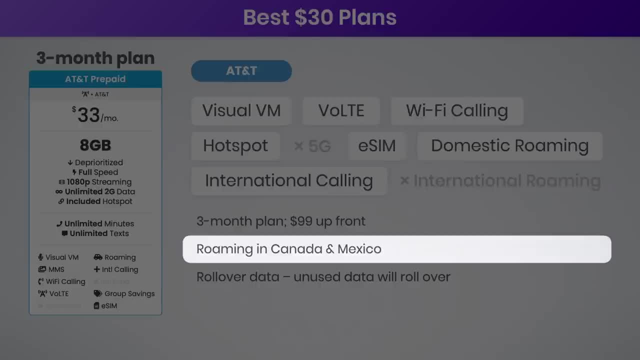 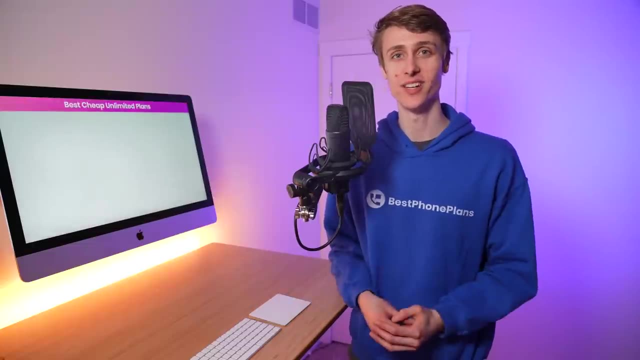 calling eSIM, domestic roaming and roaming in Canada and Mexico, as well as rollover data. Now let's move on to what may be one of the most popular categories here: the best cheap unlimited data plans. Here we have great options from Visible. 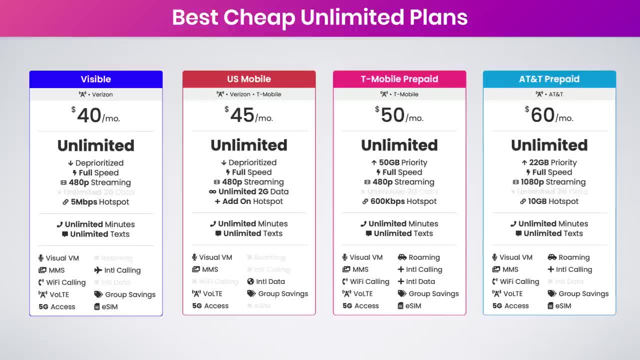 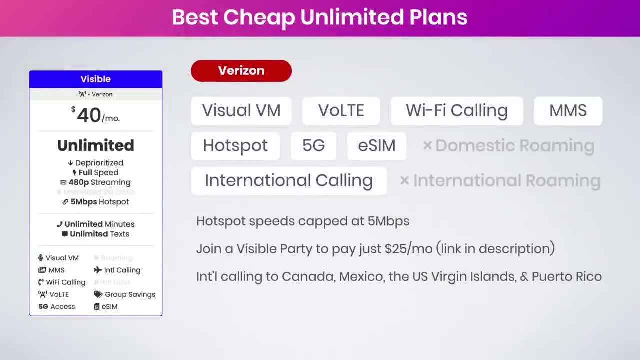 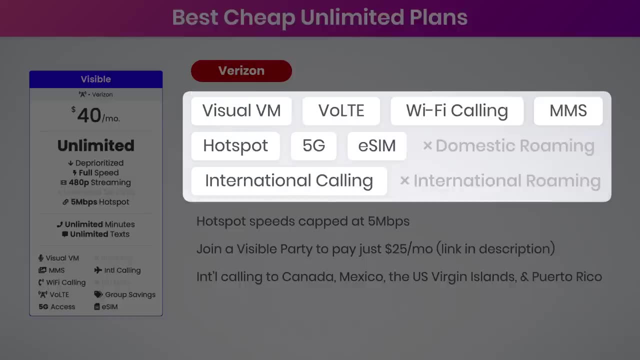 US Mobile, T-Mobile prepaid and AT&T prepaid. First is Visible's legendary $40 unlimited plan. This has exploded in popularity thanks to its excellent value, its excellent features and the fact that Visible is using the Verizon network for coverage. You get support for pretty. 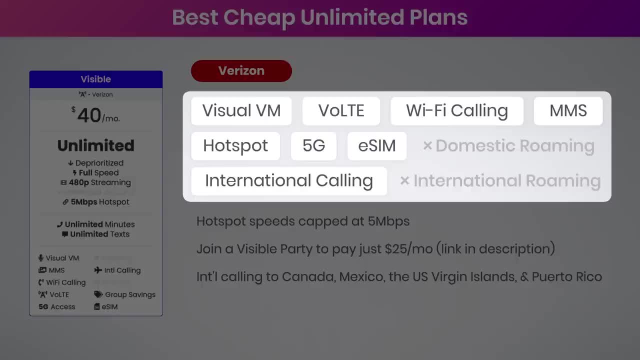 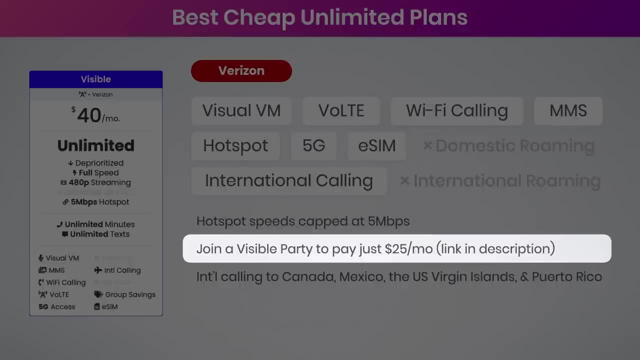 much everything here, most notably eSIM support and even 5G access. You also get unlimited hotspot data with speeds at 5 megabits per second. The best part is, if you join a Visible party, your bill will drop to just $25 per month, all taxes and fees included. If you're interested. 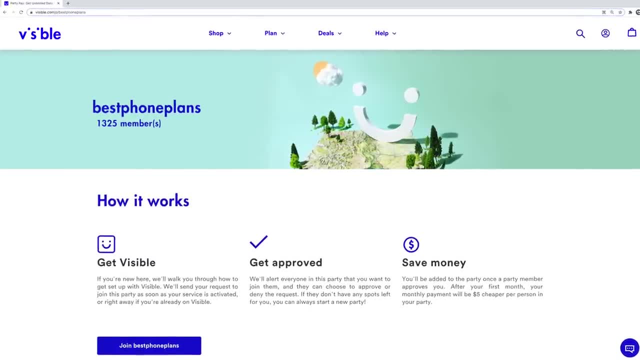 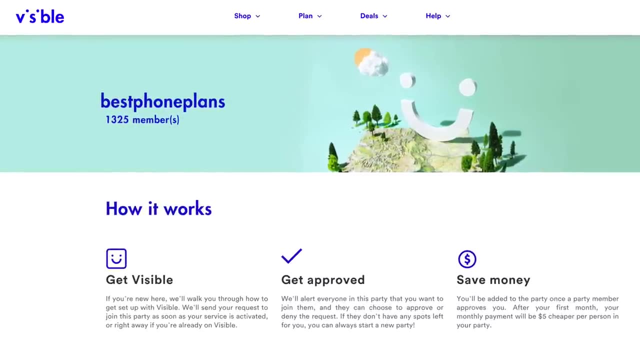 you can join my party. Best Phone Plans linked in the video description. We currently have 1,325 members and counting, and this is a great way to reduce your cell phone bill. The one downside to Visible is they don't work with all devices. 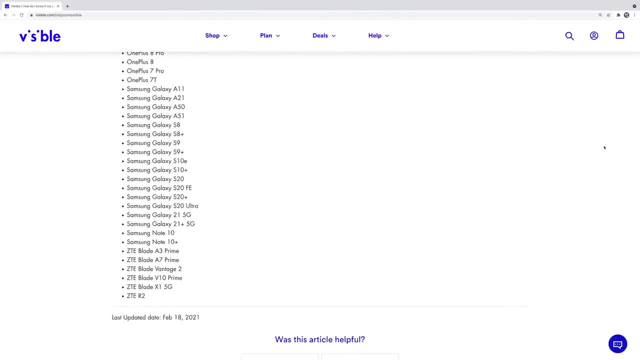 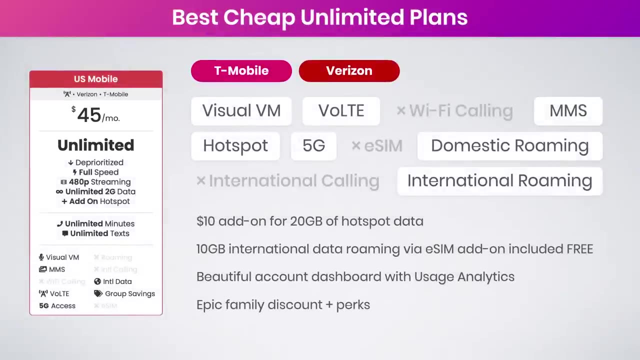 so you'll want to make sure your device is supported before you sign up. Next up is US Mobile's $45 unlimited plan. This uses either Verizon or T-Mobile for coverage, though the plan is limited to 50 gigs on T-Mobile, as opposed to the true unlimited plan. 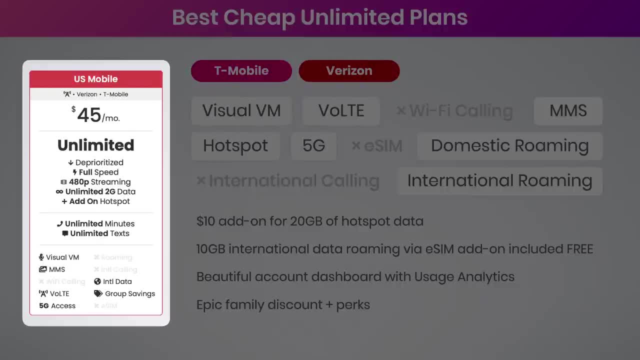 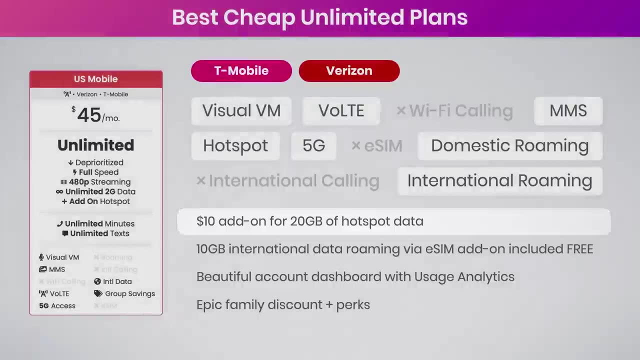 you get on the Verizon network. What makes US Mobile a compelling option over Visible, even though it is more expensive and hotspot data is a $10 add-on- is that US Mobile typically offers slightly faster speeds, better coverage and it works with more devices, as in all devices that work on the Verizon network. 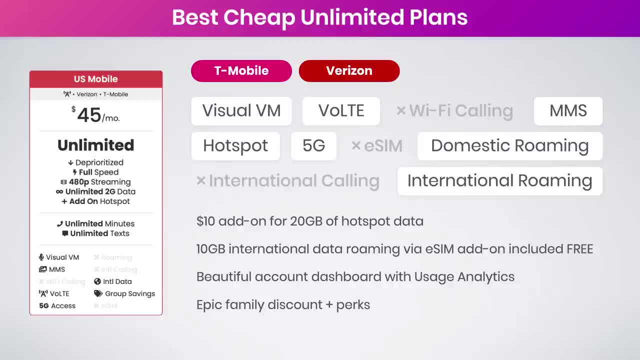 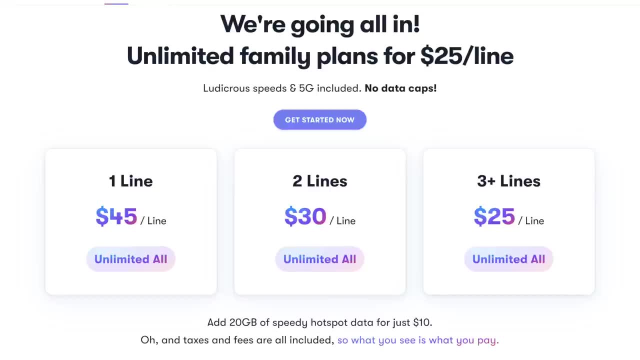 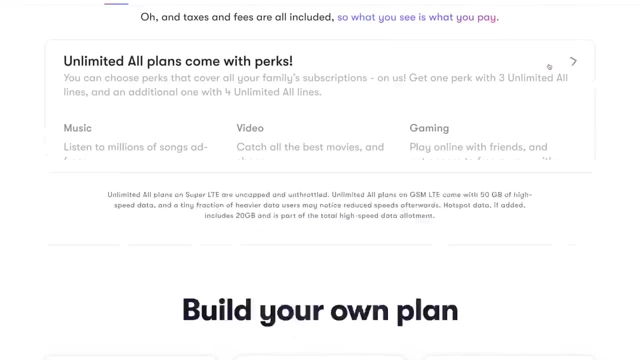 You also get 10 gigs of international data roaming included for free. Families will also love US Mobile for their multi-line discount and perks. With three or more lines, US Mobile drops the price down to just $25 per line, all taxes and fees included, and you actually get to choose up to two perks. 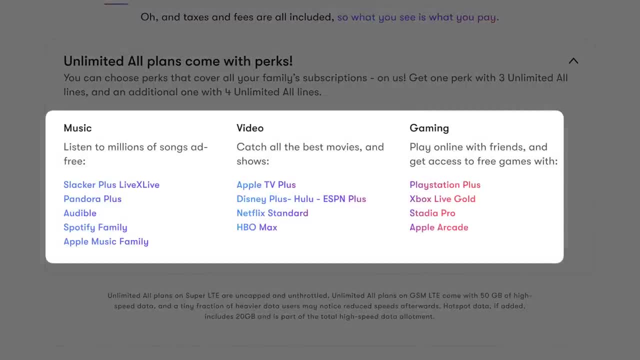 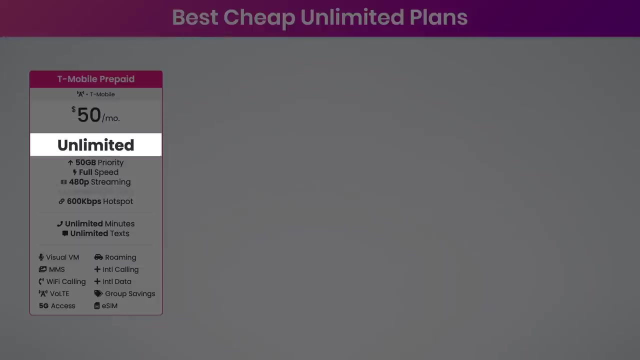 to cover the cost of your favorite subscription services. Options include Spotify Family, Apple Music Family, Disney Plus, Hulu, ESPN Plus, Netflix, HBO Max and popular gaming services. On the T-Mobile network. we have T-Mobile's $50 prepaid plan. This is a true unlimited plan. and what I love about this plan is the data is actually prioritized, so you'll have the exact same experience as if you were signed up with one of T-Mobile's more expensive Magenta or Magenta Max plans. T-Mobile also goes all out with feature support here, including things like 5G. 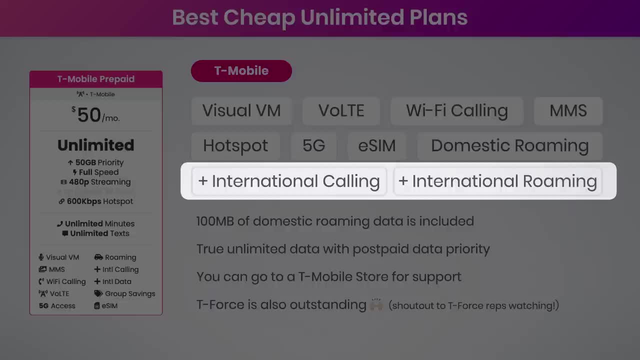 eSIM 100MB of domestic roaming data and the options for international calling and international data roaming add-ons. Finally, the other huge perk about this plan is you can go to a physical T-Mobile store for customer service and support. You can also chat with T-Mobile's T-Force. 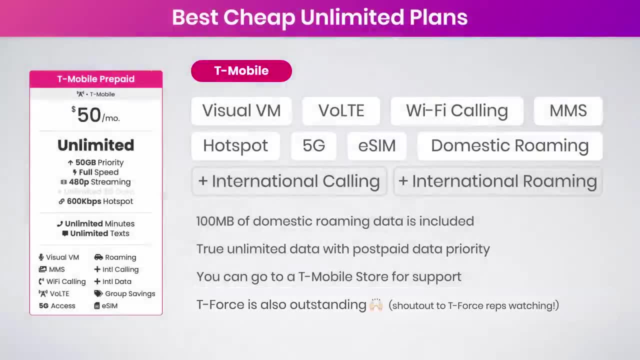 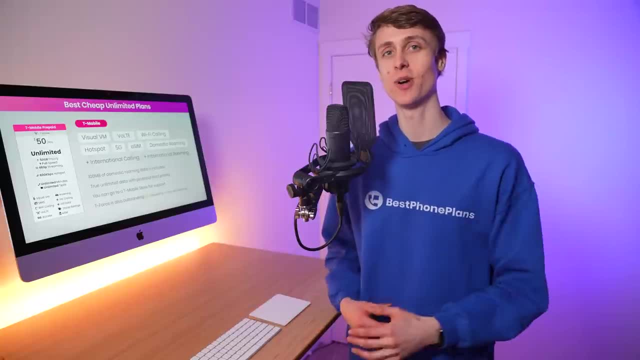 representatives on social media for help or questions about your plan, and I think T-Force representatives provide some of the best support in the world. Shout out to all of the T-Force reps watching this video now. I appreciate you and I thank you for all of your work. 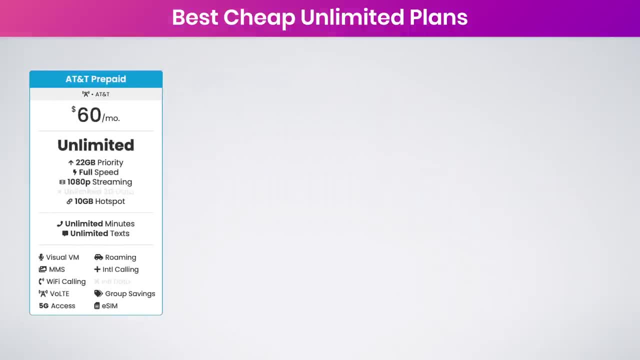 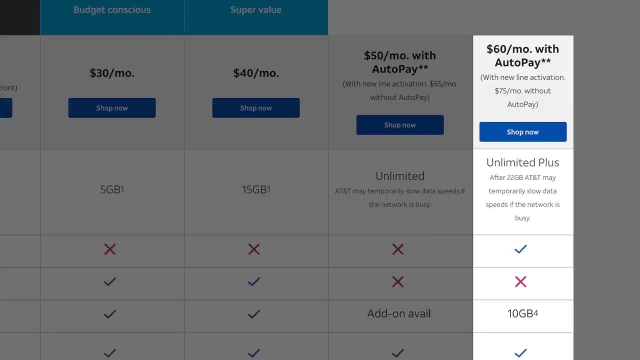 Finishing off this category, we have the AT&T prepaid unlimited plus plan. This is listed for $75 on AT&T's website, but there is a $15 autopay discount that brings the cost down to just $60 per month. This is still one of the more expensive plans I'm recommending. 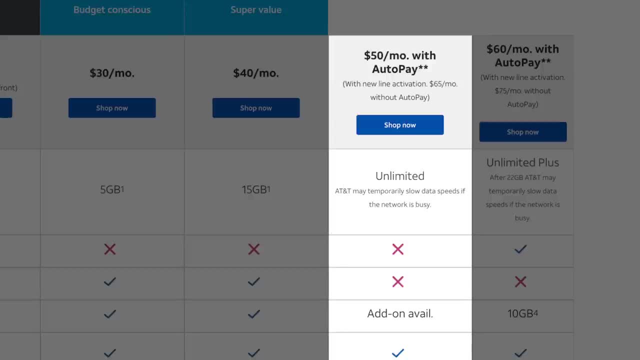 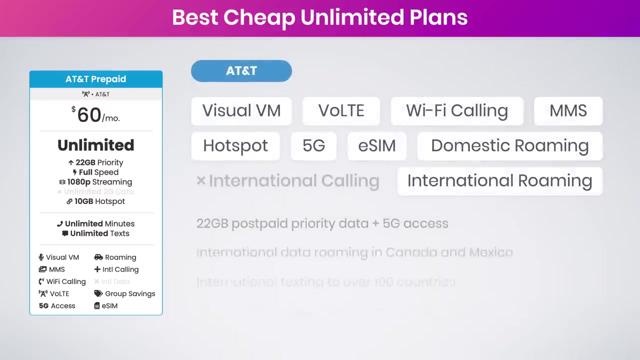 in this category, but I do think it's worth it. AT&T offers a cheaper $50 unlimited prepaid plan, but I'm recommending the $60 one because it includes 22 gigs of priority data, 5G access, 10 gigs of hotspot data and HD streaming. I think the added perks are worth. 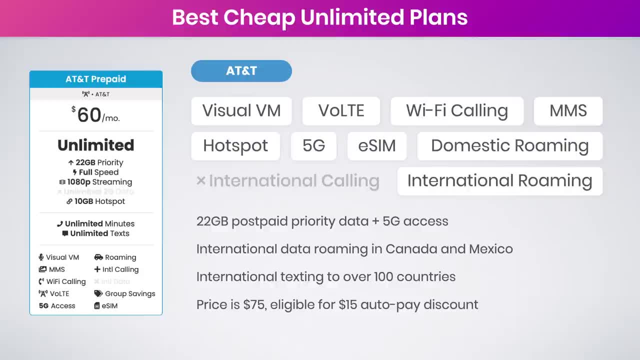 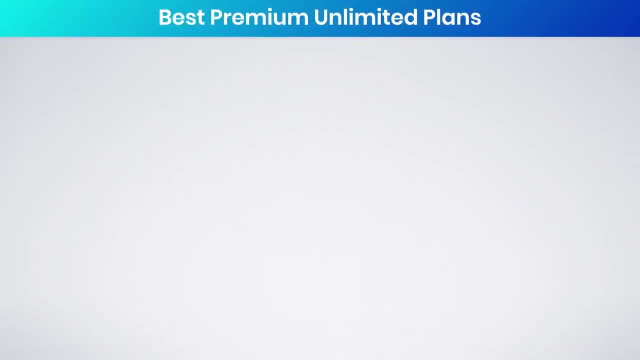 it for the slight extra cost, and this is easily one of the best value unlimited plans currently available on the AT&T network. And now onto the grand finale: the best premium unlimited plans for 2021.. I'm actually breaking this category into two brief sections. 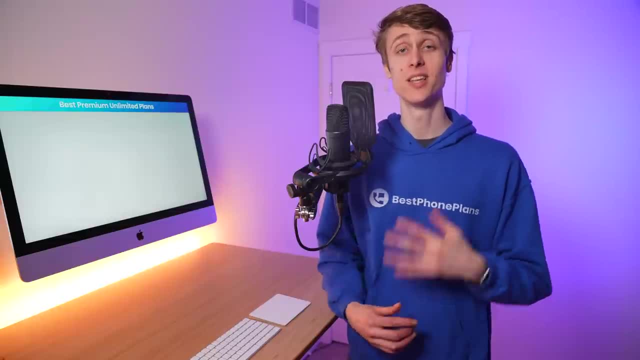 Number one: the AT&T prepaid unlimited plans. Number two: the AT&T prepaid unlimited plans. Number three: the AT&T prepaid unlimited plans. Number four: the AT&T prepaid unlimited plans. Number one: the best value premium plans that I think most people should sign up for. And number 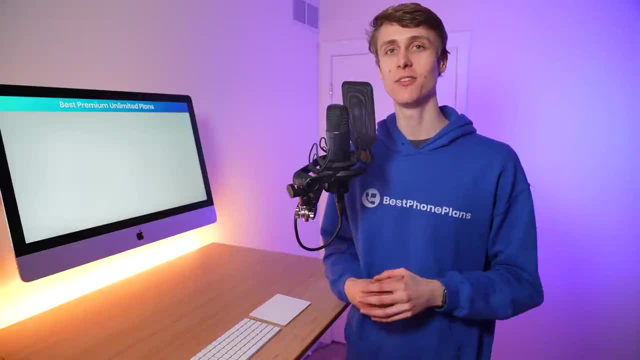 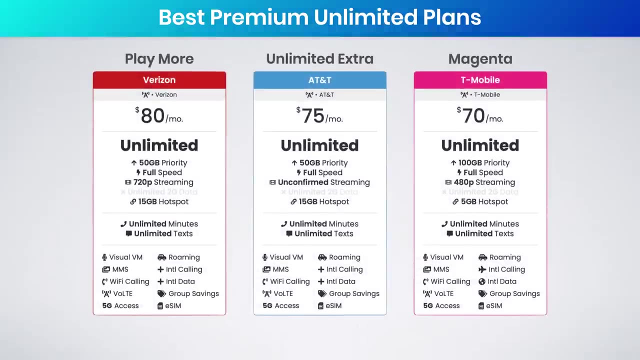 two the all-out best premium plans currently available on all the major networks. For the best value plans, I'm recommending Verizon Play More Unlimited, AT&T Unlimited Extra and T-Mobile Magenta. These come in at $80, $75, and $70 respectively And I think for most people. 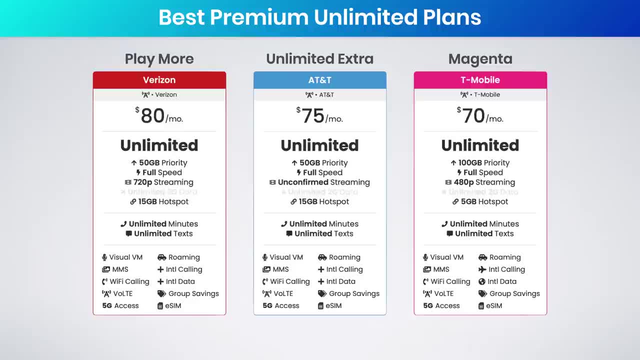 they offer the best balance between premium features and price. Though, if you can afford it and you do want to step it up a notch, you can also consider the best premium plans currently available in the industry, And those are, of course, Verizon- Get More Unlimited, AT&T Unlimited Elite and T-Mobile Magenta Max. 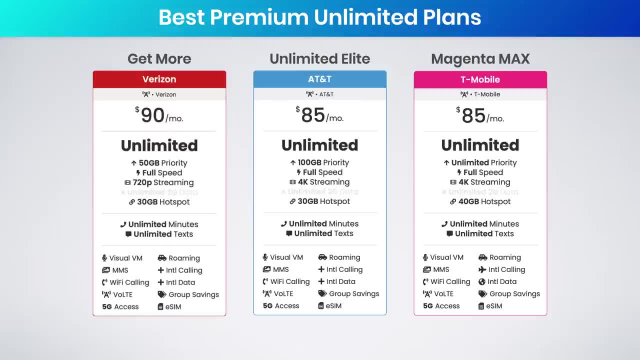 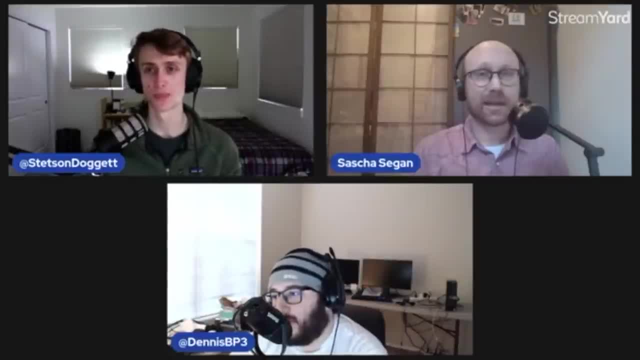 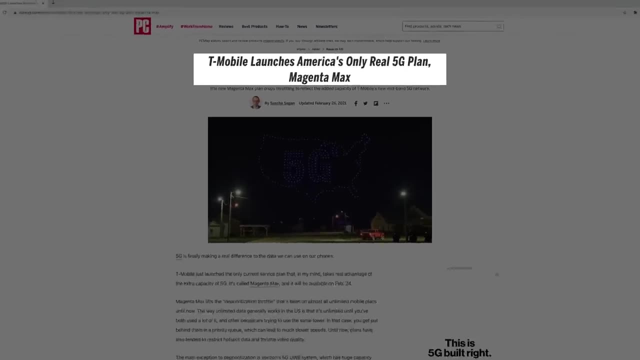 I'm surprised to say it, but T-Mobile is actually offering the most features with their Magenta Max plan. Sasha Segan from PCMag, whom Dennis and I did an interview with for our Best Phone Plans podcast, called T-Mobile's Magenta Max plan the only real 5G plan in America right now. It includes unlimited. 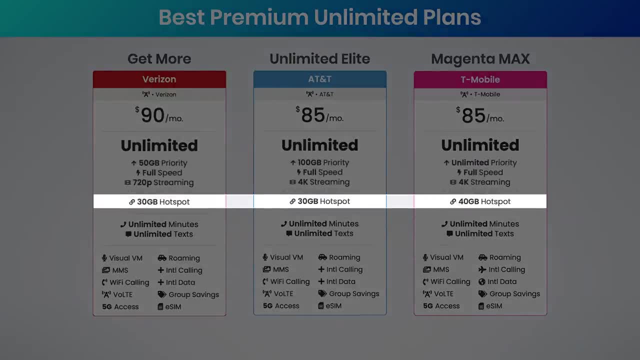 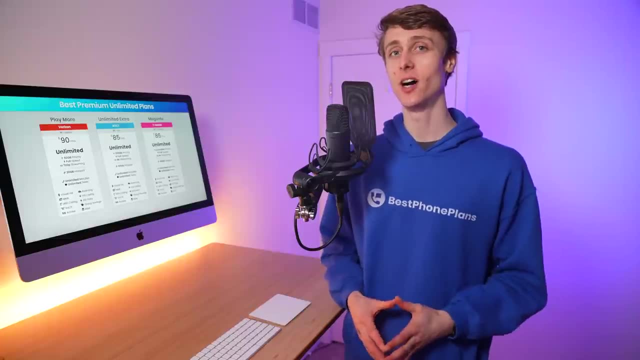 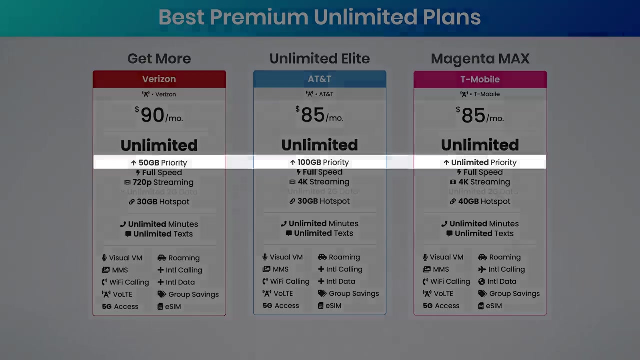 priority data: the most in the industry, the most hotspot data at 40GB, and T-Mobile's network has gotten surprisingly good recently. I also know AT&T Unlimited Elite is a fan favorite. Shout out to you, Dennis, I do know you love AT&T Unlimited Elite. It includes 100GB of priority. 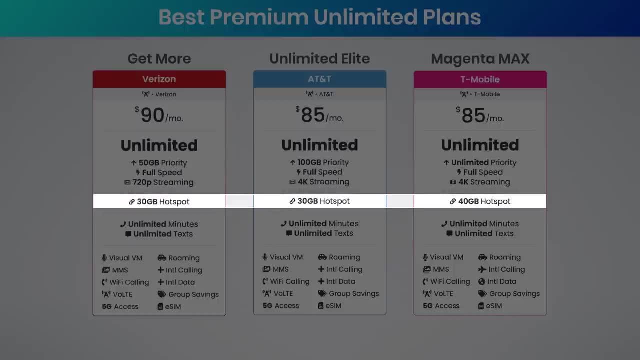 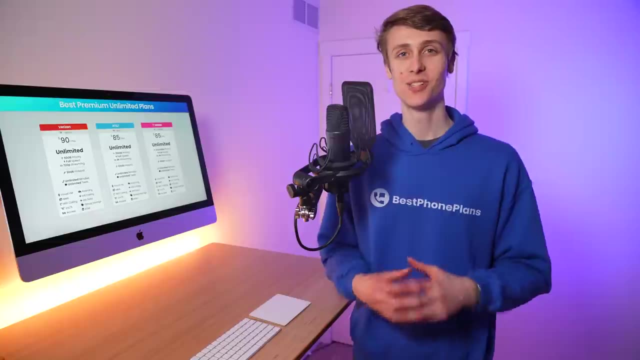 data more than Verizon, the same 30GB of high-speed hotspot data, 4K video streaming, and it includes HBO Max, which I'm told is a great perk to have. So there you go. Those are the best cell phone plans for 2021.. I spent a ton of time on this. 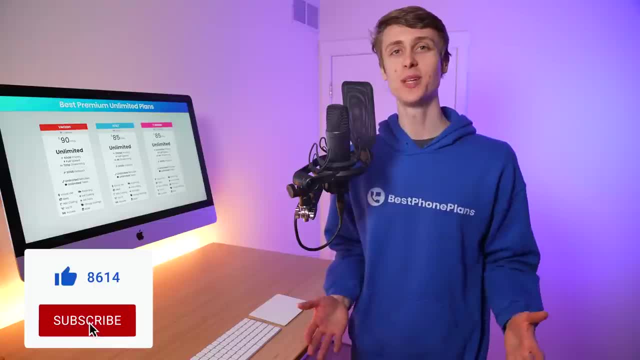 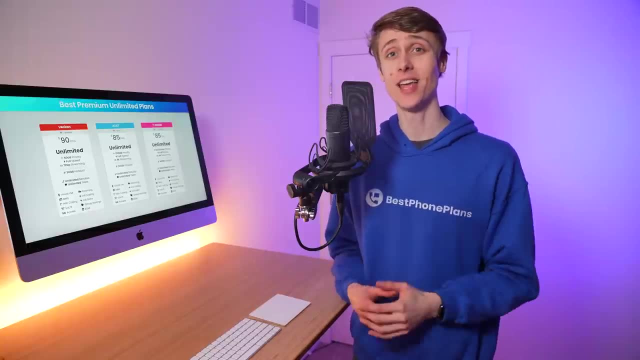 video, so if you enjoyed it or found it helpful, I would really appreciate it if you clicked the like button down below and shared this video with one friend. Also, if you're wondering how I came up with all of these best cell phone plans, I have a spreadsheet that compares over 300.